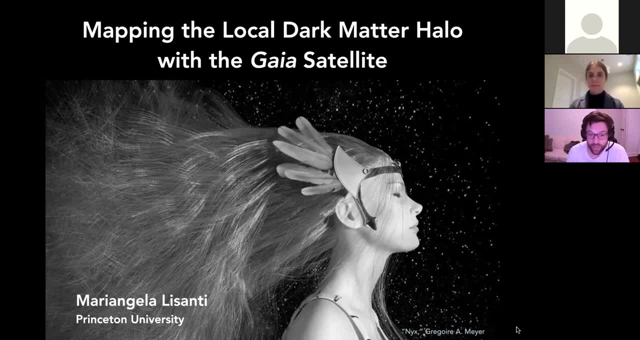 So please join me in welcoming Mariangela and, because of the online format, we're going to do questions at the end, so you know the drill. Okay, take it away, Mariangela, Thank you. Thanks so much, David, and thank you for the invitation to join you all virtually today. 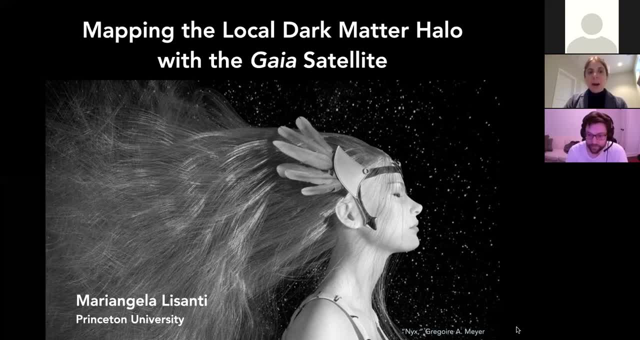 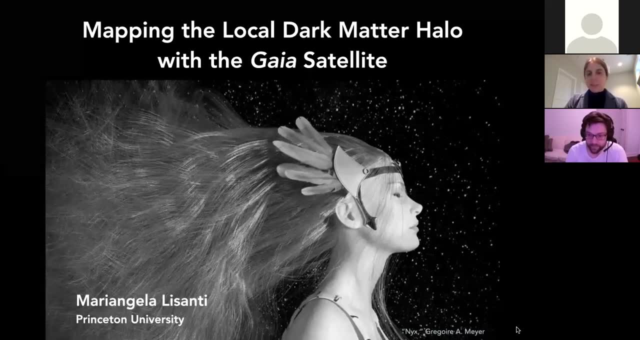 It's a pleasure to be here, So I'm starting on my. I'm starting on my opening slide here with an image of the Nyx goddess, and this is intended to be a bit of a teaser. This is a Greek goddess that will come back to our story later in the talk, so 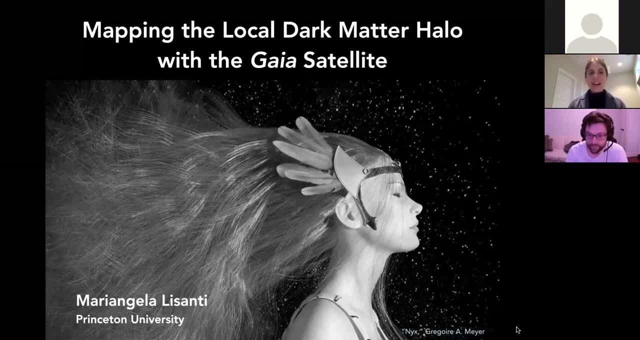 this is just kind of meant to pique your interest and that way you can kind of stay tuned to see where she makes an appearance in the story that we're going to discuss today. So what I'm going to be telling you a little bit about is some work that my group has been doing over the last 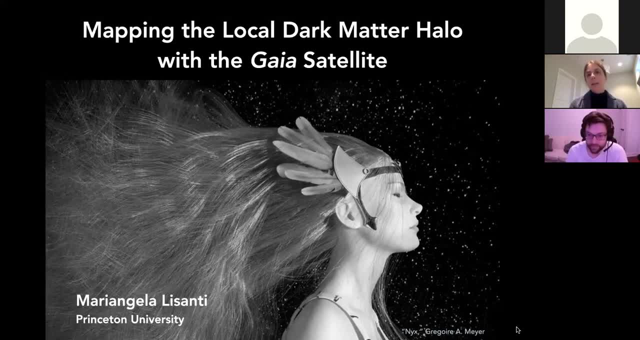 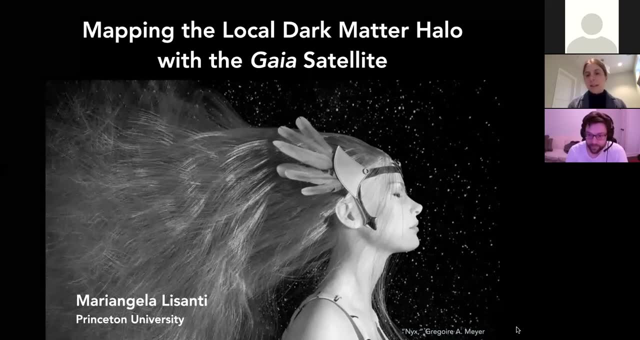 few years attempting to map the dark matter halo locally, so near the solar position in the galaxy, using data from the Gaia satellite. The primary application of this is to direct detection experiments, So these are terrestrial experiments that are seeking to discover dark matter, and those experiments rely on having an accurate map of the 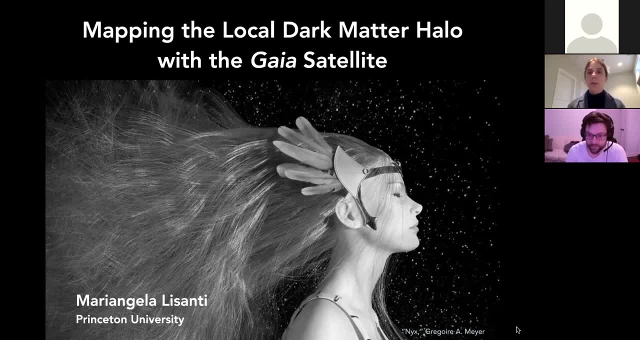 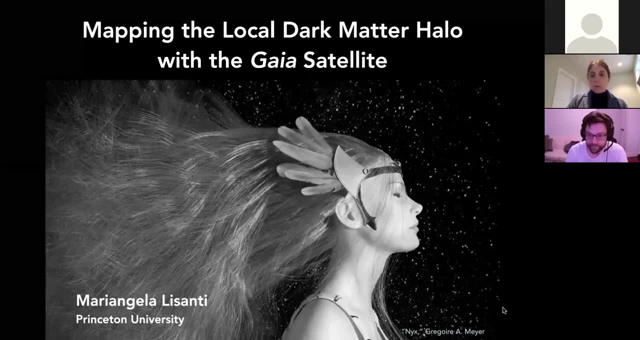 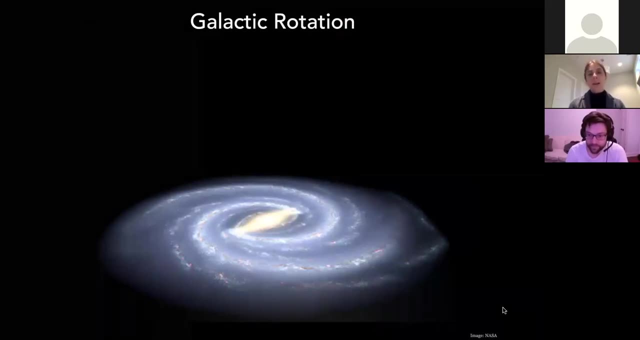 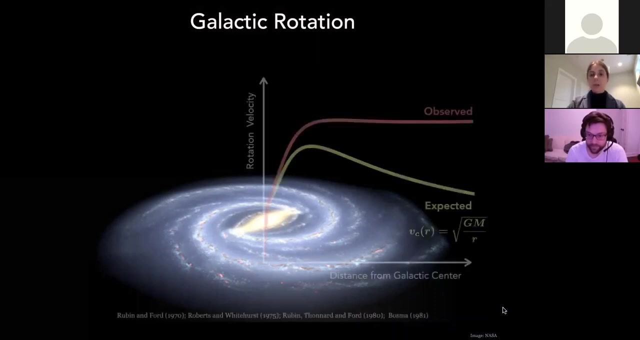 both the local number density and also the velocity distribution of the dark matter halo. So let me start by just giving a bit of a historical introduction to what we believe or have been using for our dark matter map to date, And this goes back to the 1970s and 1980s with the discovery of flat rotation curves. 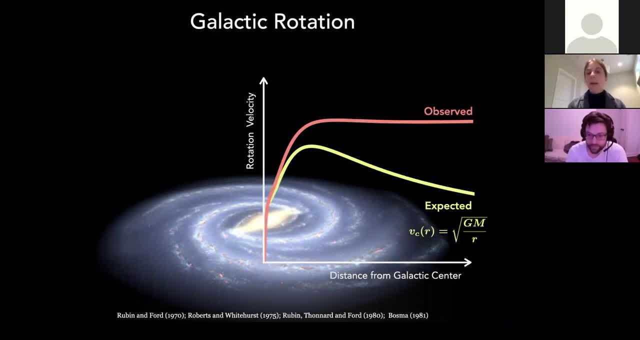 Where we, you know, with work pioneered by Rubin and Ford, saw that the rotation velocity of galaxies similar to the rotation velocity of stars, where we, you know, with work pioneered by Rubin and Ford, saw that the rotation velocity of galaxies similar to the rotation velocity of stars. 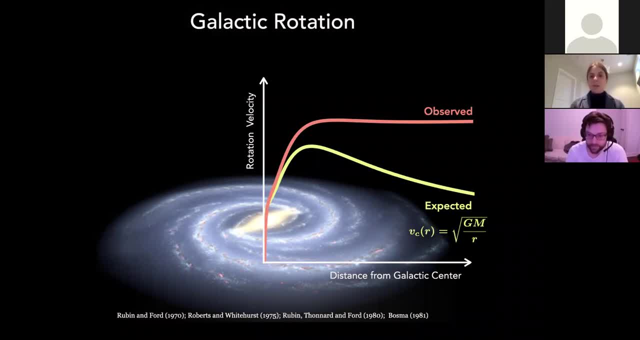 similar to ours, flattens out at large distances from the center of the galaxy, which is different than what's expected from the Newtonian prediction. There are several ways that you can explain this result. One way is to posit that the Newtonian gravity itself as a theory is failing, and that we need to modify gravity in order to explain this. 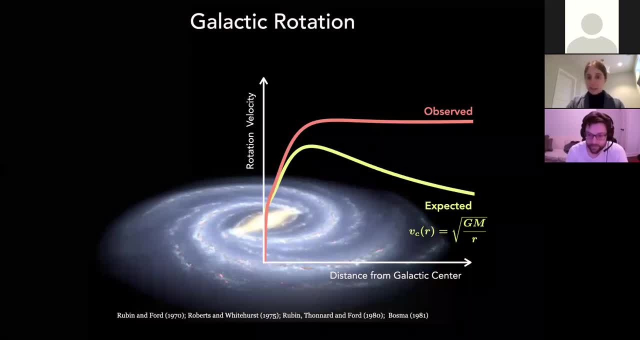 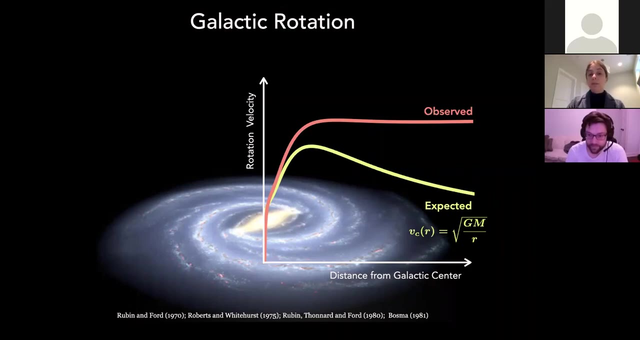 And modifications to gravity have received a bit of attention over the last few years. They struggle. the models that have been posited struggle to be able to explain cosmology, cosmological signatures like the CMB. so that's been one of the primary challenges to at least the models that have been developed to date. 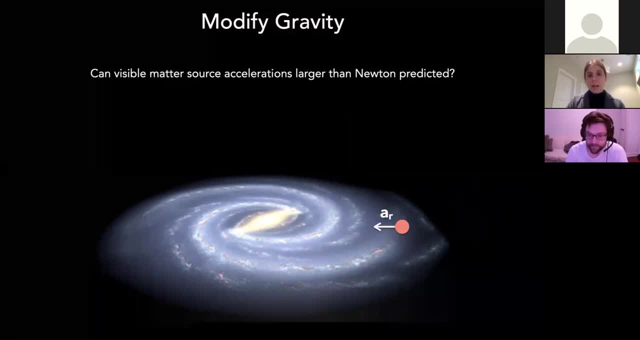 My group recently did another test of MOND-type modifications to gravity, looking more locally within our galaxy, Precisely in the range where these kinds of models are predicted to be modified, And we found that both of these modifications were most successful. And what we were looking at was comparing the radial accelerations of stars versus their vertical accelerations. 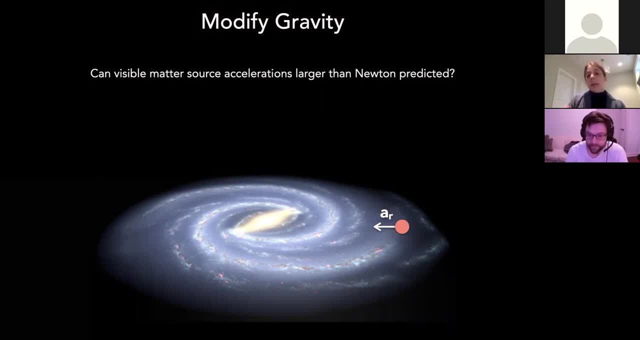 What modifications to gravity do is essentially enhance the radial accelerations of stars such that at far distances to bring them in line with the flat rotation curve results. But when you do this, the theory also simultaneously enhances the vertical acceleration of stars. So we can actually just go into the data and see whether those enhancements in the vertical accelerations exist. 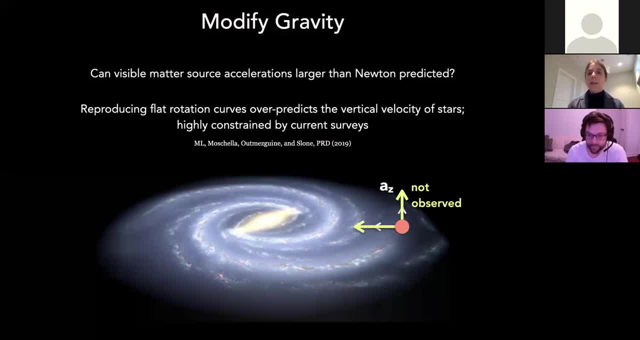 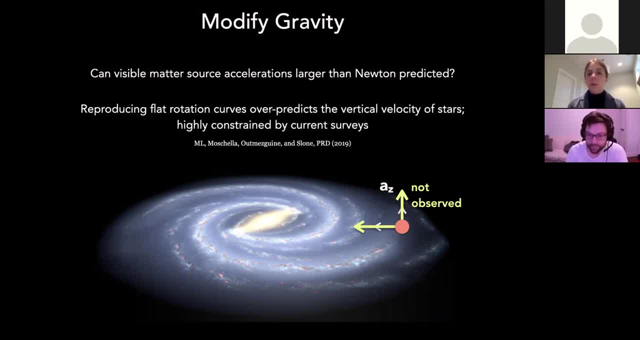 So I think that's what we're looking at. So I think that's what we're looking at Precisely in the region where these models are supposed to be successful. So what that leaves us with, then, is the second approach to explaining flat rotation curves, which is that we introduce additional mass in the galaxy. 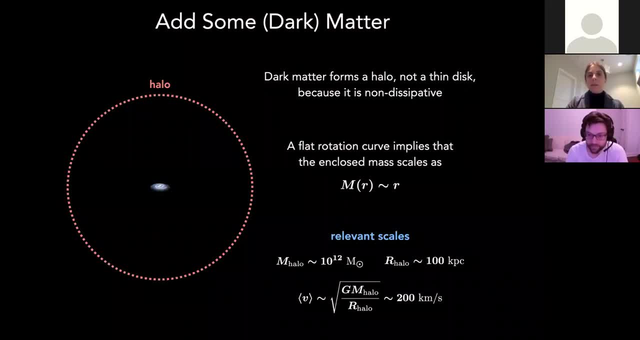 And in this framework, we can think of this as additional- let's call it dark matter. So it's additional matter that's not emitting any light And it surrounds the visible part of our galaxy in a very massive halogen halo. The extent of this halo is far, far greater. 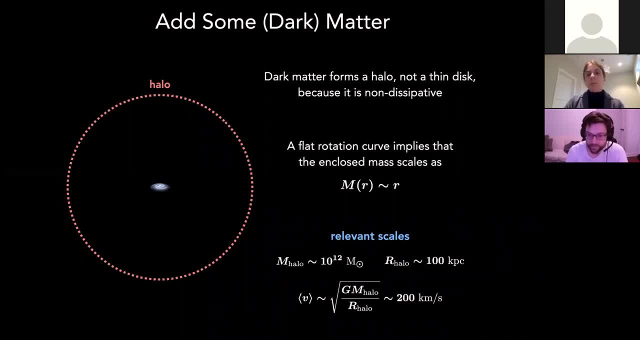 than the extent of the visible part of the galaxy. Specifically, you can think of the radius of this halo as being nearly 10 times the radius of the baryonic halo. The dark matter particles that would be flying around in this halo are, in some sense, pretty boring. 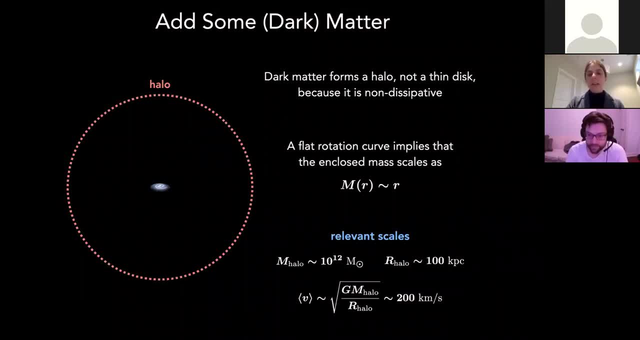 They don't really. they're not moving around at relativistic speeds or anything like that. Their average velocity is probably close to about 200 kilometers a second, And just the overall mass distribution in this halo needs to scale linearly with radius in order to be able to explain the data from flat rotation. 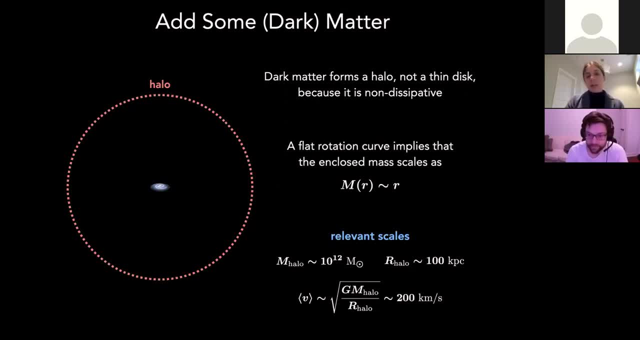 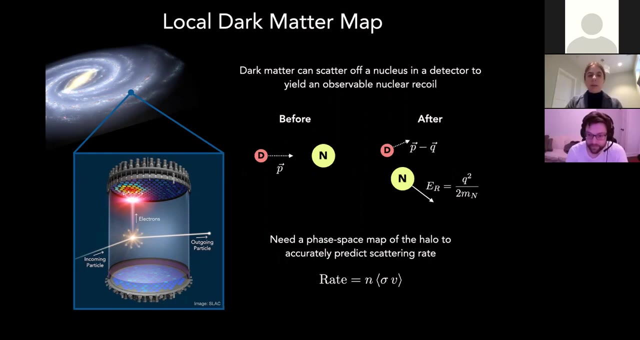 curves. So this picture taken together is one way in which we can explain the flat rotation curve data And for the purposes of any experiment where we actually really want to be able to directly detect these dark matter particles so that we can actually say something about its particles. 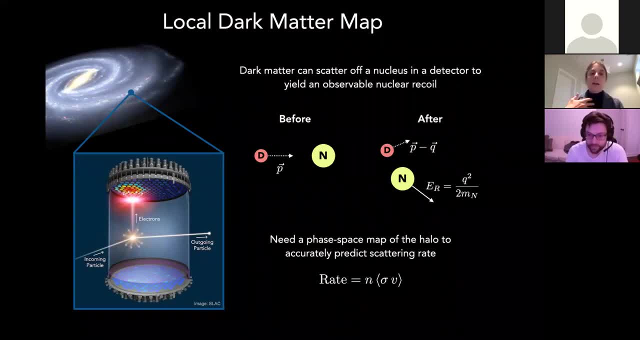 we want to be able to actually see the particle properties. So, for example, what is the mass of the particle? How does it actually interact with visible matter? In any of those kinds of experiments, we want to be able to actually see the interactions of these particles. 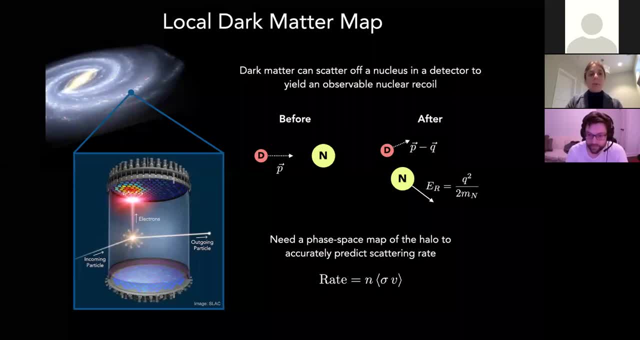 let's say, in a terrestrial experiment, some lab here on Earth. For example, in the diagram, the image I have here on the left, this is an experiment called Xenon 100.. At the moment they're running a much larger version, Xenon 100. 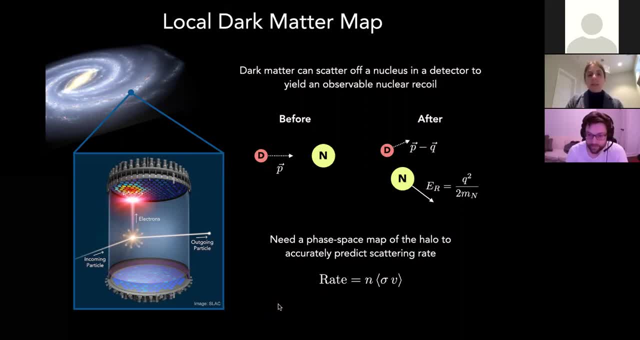 It's essentially just a big tub of Xenon And what the experiment is doing is essentially waiting for a dark matter particle to fly through, collide with the nucleus in that detector. The dark matter particle is obviously never going to be observed, but the recoil energy. 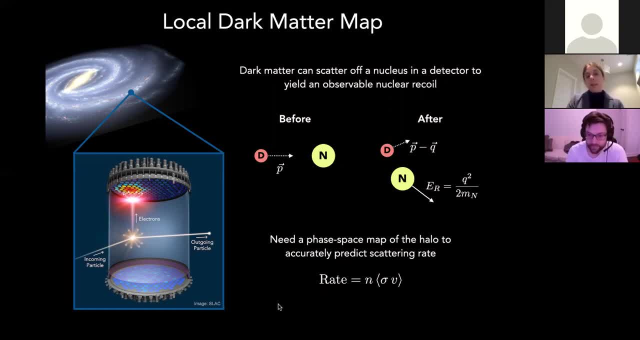 that it imparts to that nucleus leads to a signal that can be detected. Now the scattering rates in any of these kinds of experiments are going to depend on the phase space of the local dark matter. So, as I said earlier, both on the number, density. 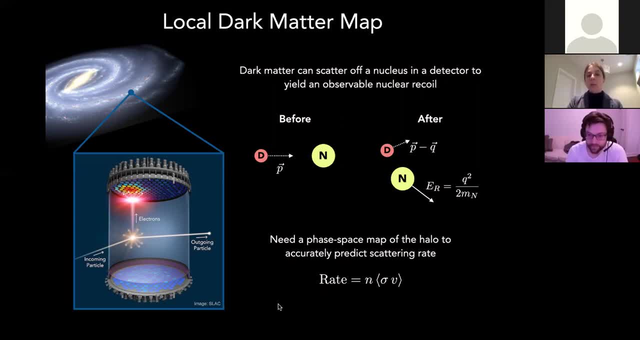 of the dark matter in our corner of the galaxy, as well as the velocity distribution of the dark matter in our corner of the galaxy. And these two uncertainties are perhaps one of the two largest systematic uncertainties that come into play when interpreting the results from these direct detection experiments. 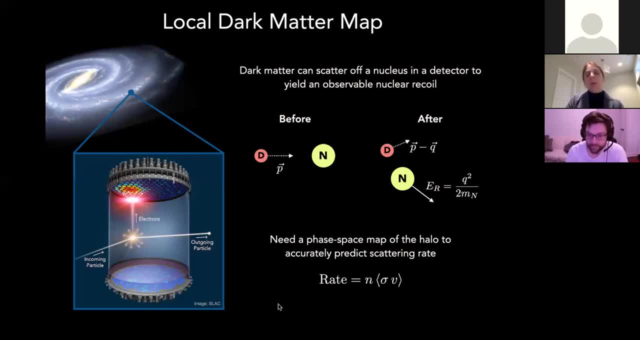 So if we can get these uncertainties better under control, it would ultimately end up helping us to decipher the actual fundamental properties of dark matter from the galaxy. So that's what we're trying to do. We're trying to find a way to do that. 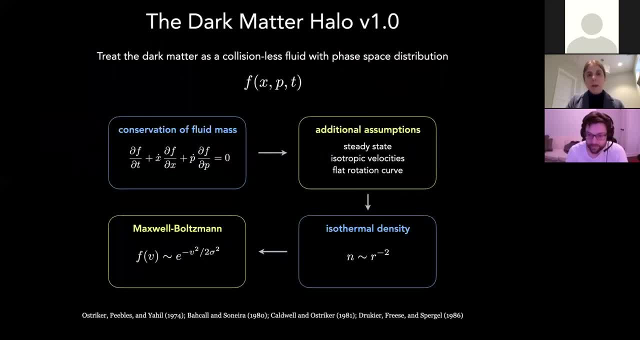 And we're trying to find a way to do that- from any possible signal that we would record The sort of the history for actually writing down a model for that local dark matter. number, density and velocity distribution follows pretty closely on the heels of the discovery of the flat rotation curve. 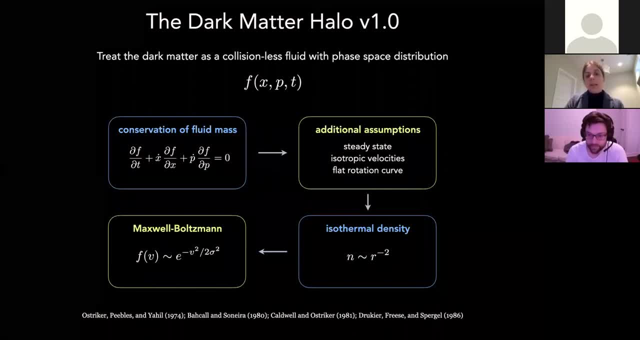 So this is in very early work by Ostreicher and Peebles in the 1970s and then Fries and Spergel a little bit later than that. And the goal here is: how do we actually write down a model for this dark matter? not really. 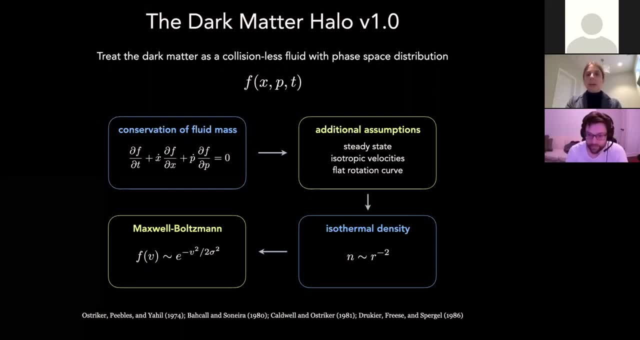 knowing too much about it. So we'll assume that it's a collisionless fluid and that the fluid mass is conserved. So that's this initial assumption in this blue box here, And then, if we add onto this a few other assumptions, so for example, we state that this dark matter is: 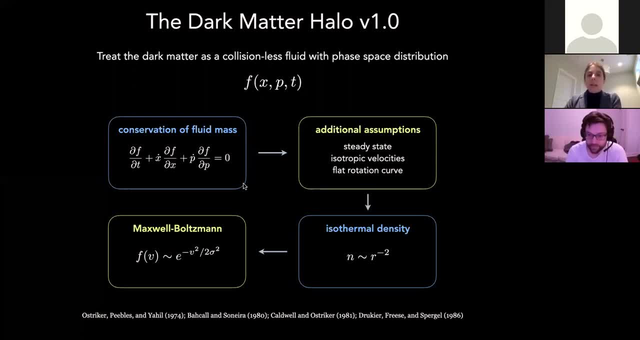 in steady state, that its velocities are isotropic and that it ultimately would end up explaining a flat rotation curve. Then, taking these assumptions and combining it with the conservation equation, what falls out is that the number density of the dark matter is 1 over r squared and that its velocities are just. 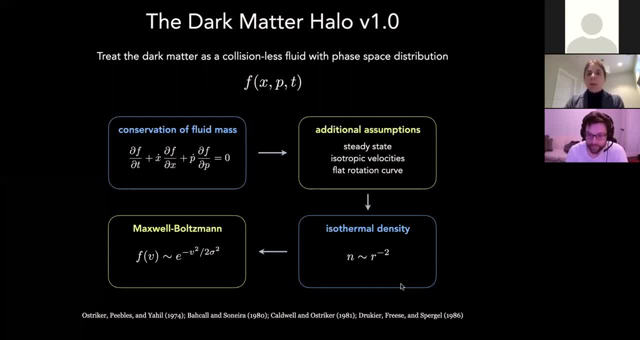 simple Maxwell-Boltzmann distribution. So this model was put forward very early on and has essentially become the standard in the field. It's actually referred to as the standard HALO model. Any result from a direct detection experiment that you see utilizes this model. 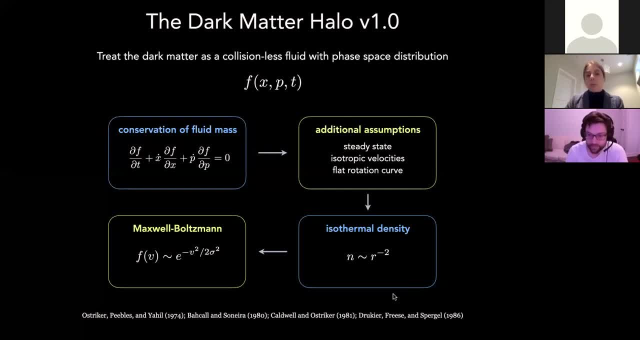 And the results, the limits, are always presented, assuming, for example, this Maxwell-Boltzmann distribution. What we have now is, with new data that I'll be describing, an opportunity to revisit this HALO model and understand whether or not the assumptions that go into this model. 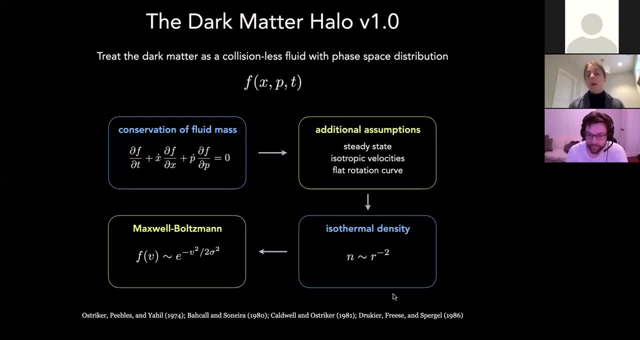 are actually the correct assumptions to be making and then also understand what the modifications of the model would be if you alter those assumptions. So, specifically, what I want to do is focus on the assumption of steady state. So what does it actually mean for a galaxy? 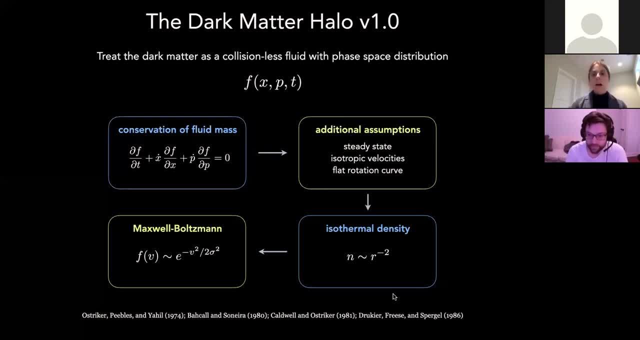 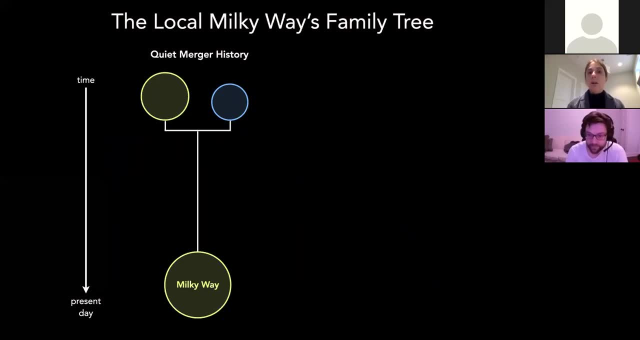 like the Milky Way to be in steady state. The way I like to think about it is in terms of the historical evolution of our galaxy. In the cold dark matter framework, galaxies like the Milky Way grow by collisions with other smaller galaxies. 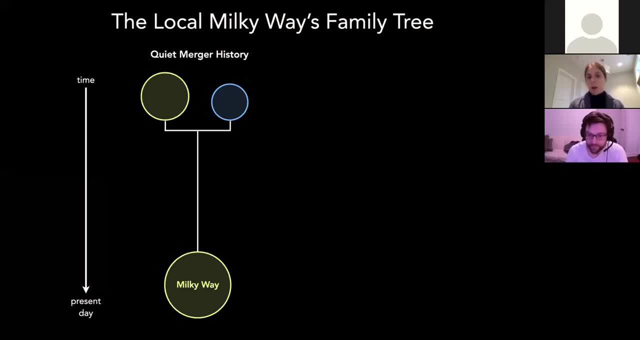 So in some ways, like beginning at the Milky Way way, of sort of having eaten up smaller galaxies and as it does it inherits the dark matter and stars from those galaxies and it grows larger and larger over time Now that merger history. so the the way in which the historical evolution, by which you've had these collision events, 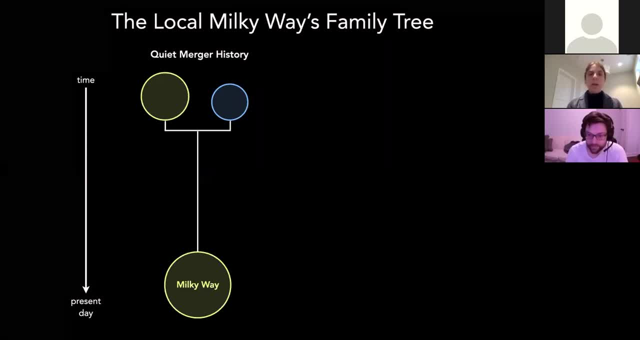 you know we can have, we can consider two separate extremes for that. so in one extreme, where the history is pretty quiet, we have first, let's say, a collision event: a long long time ago, two galaxies combined and then they just kind of settled into place and had a long time to just sort of sit there. 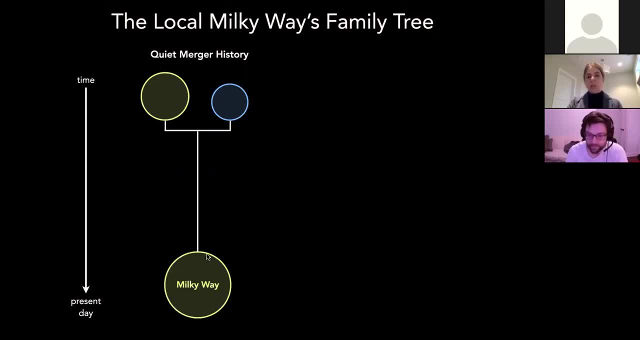 come into equilibrium. and then here we are today with our own, you know, Milky Way galaxy, and we can contrast this to a much more active history where a lot of galaxies would have combined over time, giving us our Milky Way today, and in the first case, here on the left, where are the Milky Way? 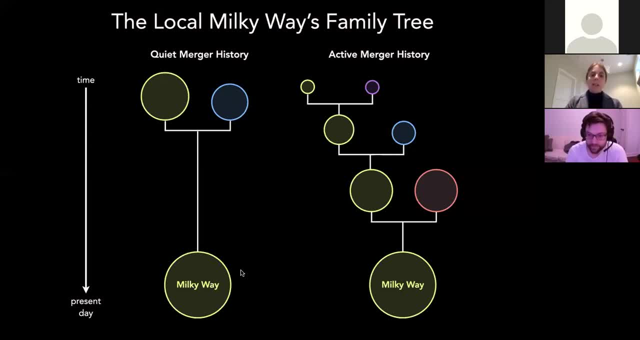 has a chance to sort of come into equilibrium over time. that's the limit where the steady state hypothesis would be correct and where the derivation that I showed on the previous slide would would fit well with the picture. but if we have a much more active merger history as depicted, 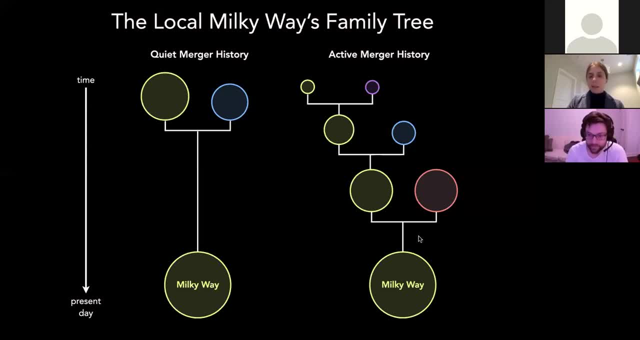 here on the right. that would challenge that steady state assumption and bring into question the, the model that we've been using all these years. So you know our, our need to be able to describe the local dark matter. history actually requires us to understand a much bigger problem, which is: how does, how does our, our galaxy actually evolve to the 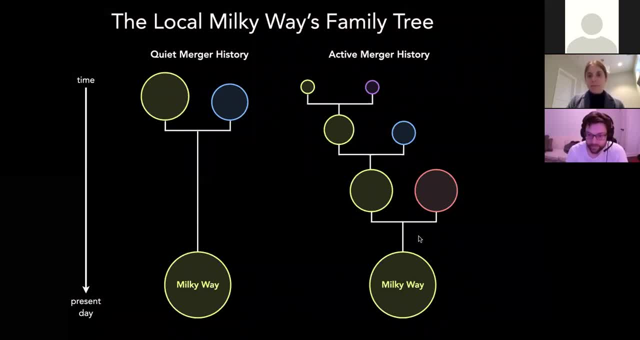 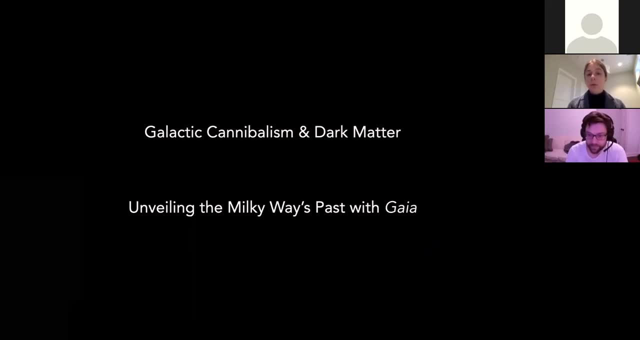 point that we that we see it today. So over the course of this talk I'm going to discuss that and also show what we've been able to learn with data from the Gaia satellite. The first part of the talk is going to focus more on the theoretical foundation for how to interpret the Milky Way. 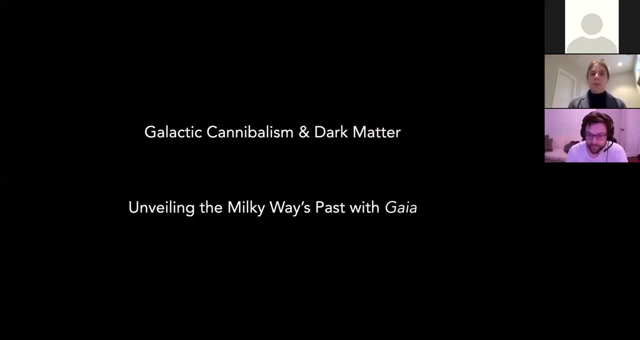 So I'll be showing you some results that we've obtained using numerical simulation and walking you through what actually happens to the dark matter as two galaxies collide in, let's say, in the Milky Way, And then, in the second part of the talk, I'll walk you through the kinds of analyses. 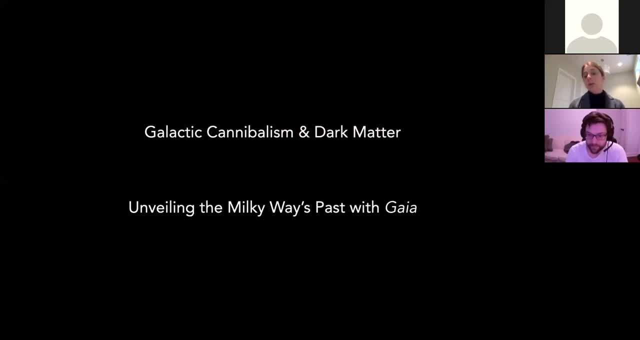 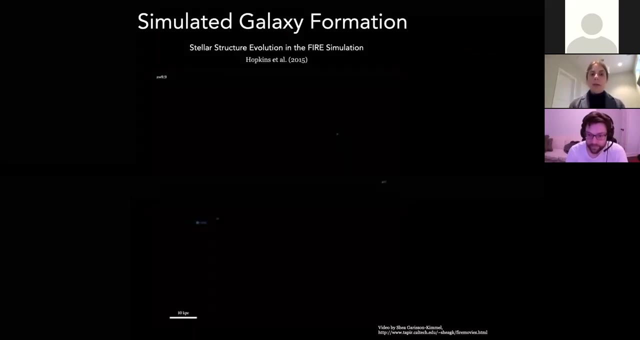 we've been doing with Gaia, to actually reconstruct our galaxy's history and be able to say something about the dark matter map near near the Milky Way. So let me show- start by just showing you- a movie of a galaxy that's similar in mass to the Milky Way. 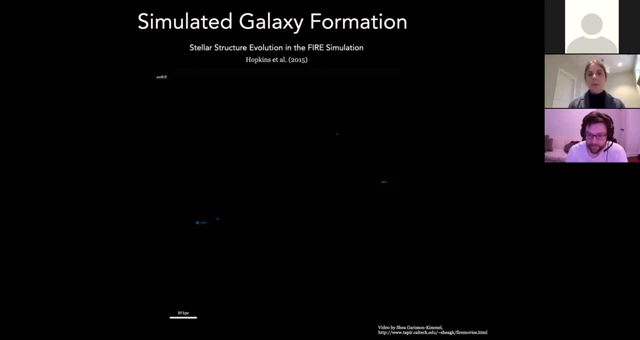 This is modeled using the FIRE simulation, where FIRE here stands for feedback in realistic environments. So this simulation tracks both the dark matter, the stars and the gas in a galaxy of similar mass to ours, starting at very low altitudes. So this is very early times, all the way up until the present day. 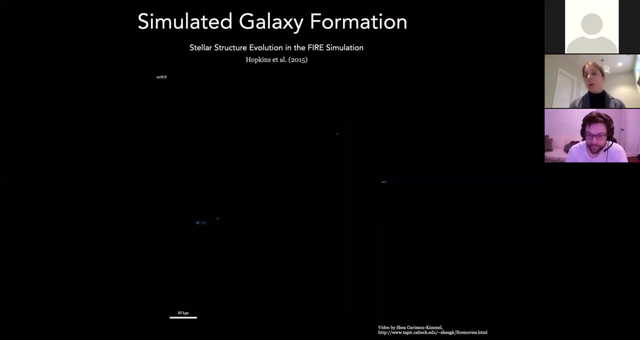 The movie that I'm going to show you only will show the stars in. you know sort of where the stars are in this process, But just keep in mind that the simulation is also simultaneously keeping track of the dark matter. So let me get get this running. 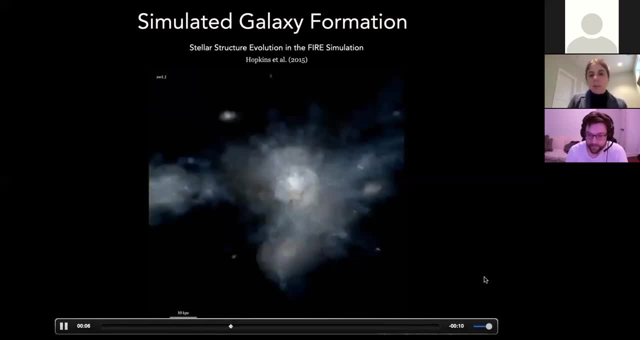 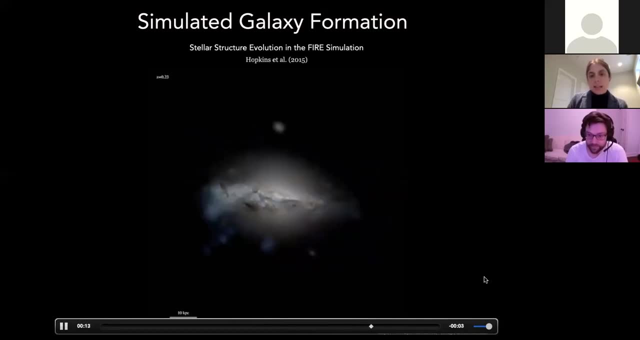 I'll run it through once and then kind of come back and highlight some, some of the points. So we're nearing the end here and in this last phase you can see you know here's the stellar disk and there's not really that much activity. But if we rewind this back and watch this again in 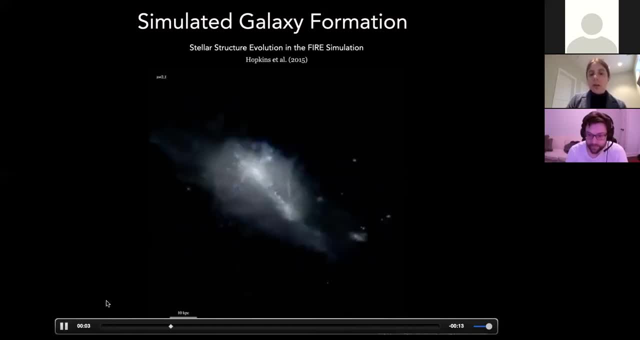 the initial stages the process is pretty violent. so you're getting a lot of these collisions and a lot of materials kind of getting stripped and moved around. it's pretty chaotic and here later on in time the number of these little mergers reduced a lot. They become smaller and that disk is is more stable so it actually survives with time. 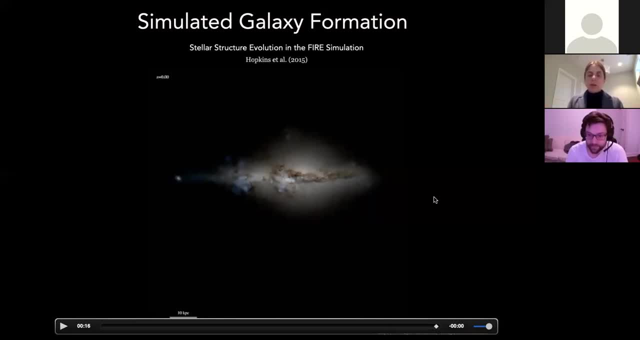 So what I want to do now is just kind of break this down, starting from, you know, kind of step by step. So, as I have one of these satellite galaxies falling in, what actually happens to the dark matter and the stars in that system and how does that evolve as I let the system? 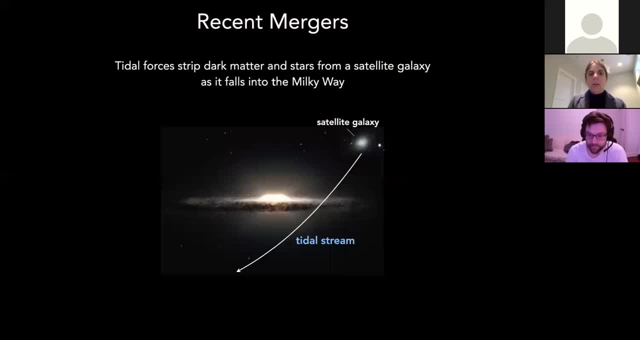 as I let time progress, So let's start off just in that initial point. So I've got my galaxy, my Milky Way, so that's represented diagrammatically here by this disk, and there's a little smaller satellite galaxy that starts falling in, so it's gotten caught by the tidal pull of our, our galaxy. 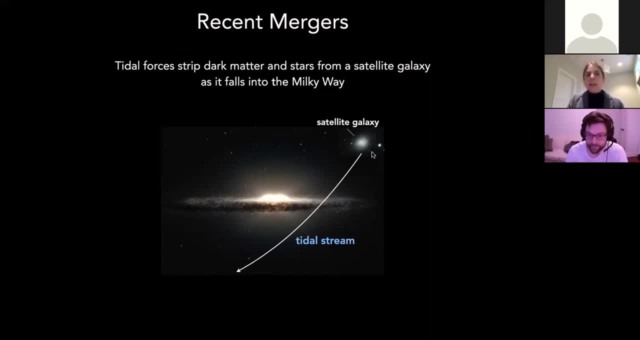 In the initial stage. as this satellite galaxy starts falling in, it is going to experience the gravitational force from our larger Milky Way and these tidal forces are going to be stripping the dark matter and the stars in that satellite galaxy off of the galaxy. The material that gets stripped off is just left behind. It's essentially just. 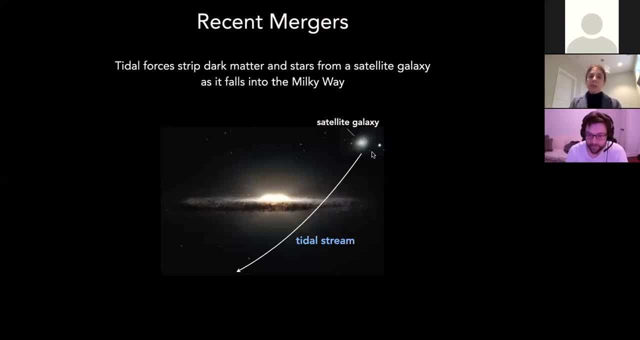 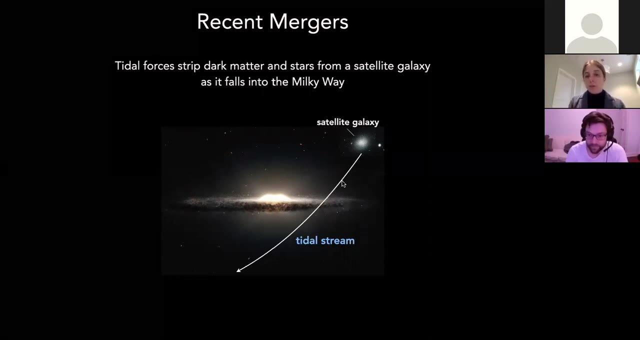 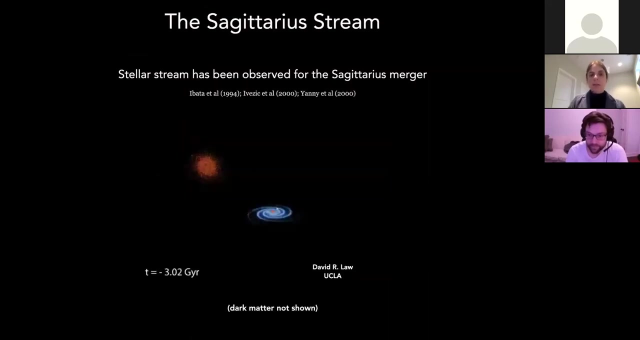 kind of litters our own galaxy and in the initial stages it very roughly kind of tracks the path that the satellite galaxy took as it falls in. This leads to essentially a tidal stream that forms, and we see evidence for these tidal streams in the Milky Way. Perhaps the most famous of these is the stellar stream. 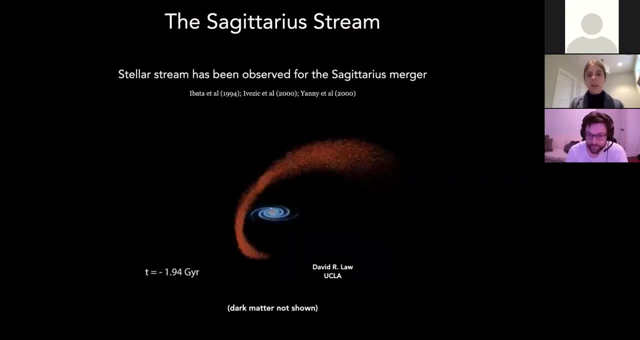 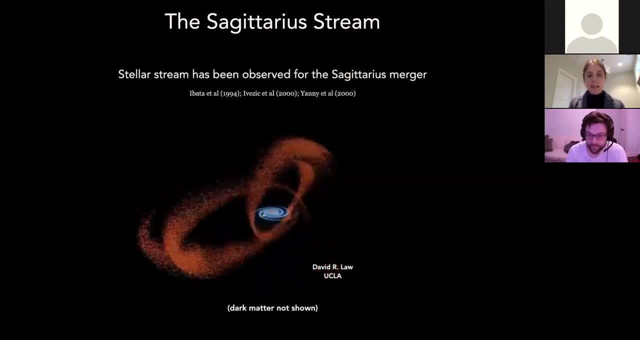 that's left behind by the merger of the Sagittarius dwarf galaxy. So this is just a movie of that merger happening and in the case of Sagittarius, the dwarf itself actually has not been completely disrupted, so we can still see the dwarf in its current position. but we can also make out these: 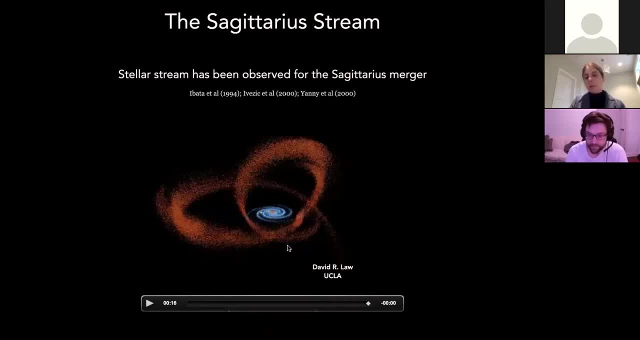 wings of the tidal stream that it has left behind. So this is just a movie of that merger happening. So in this movie the actual Sagittarius is roughly around here and you know, if we could evolve this further in time, Sagittarius will ultimately just end up being completely disrupted. but it hasn't. 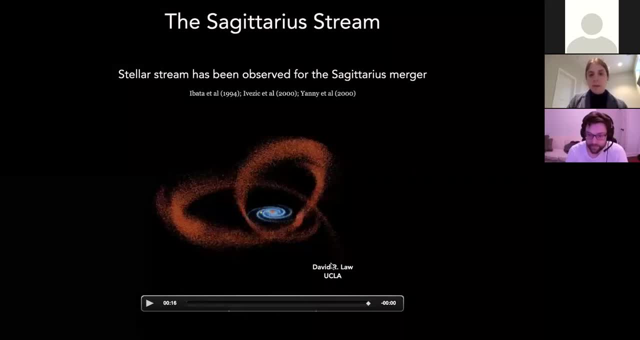 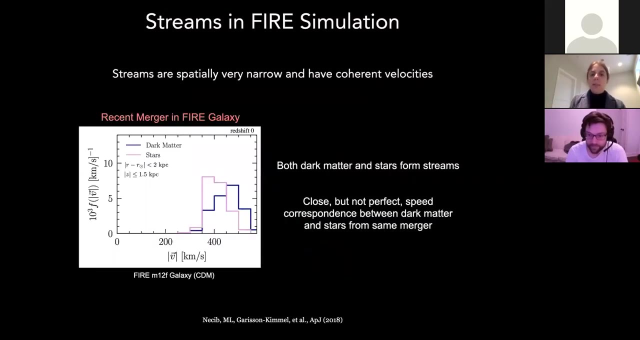 quite reached that point yet. So tidal streams are a pretty spectacular signature of these kinds of mergers. They tend to occur pretty, you know, like, as I said, like pretty soon after the galaxy starts falling in, If we consider a point in time a little bit later, once the satellite galaxy falls, 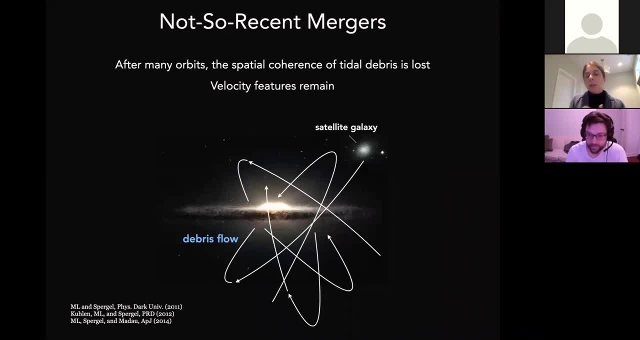 in and then makes several different orbits. you can think of this as essentially winding up all of those streams that it leaves behind, and with time, the beautiful, very clean signature that you see of a single stream essentially gets washed out and what's left just looks like kind of a cloud of. 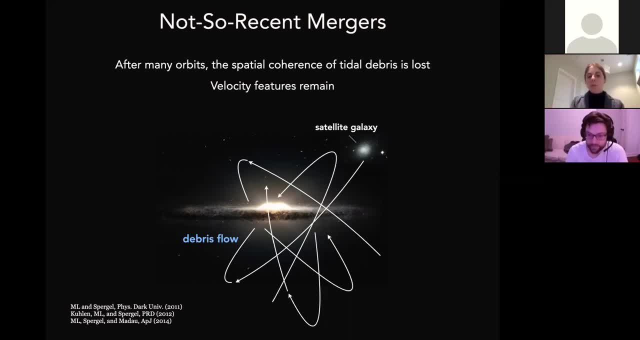 tidal debris that's left behind And what's you know, even though spatially that material does not have anything you know interesting. there aren't really that many interesting features that are there spatially. What's interesting is that the velocity behavior of the material left behind can still have some 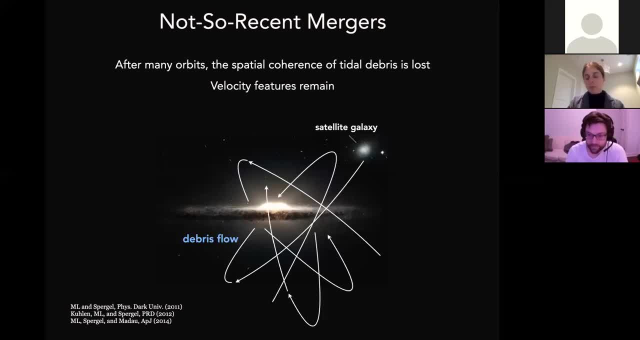 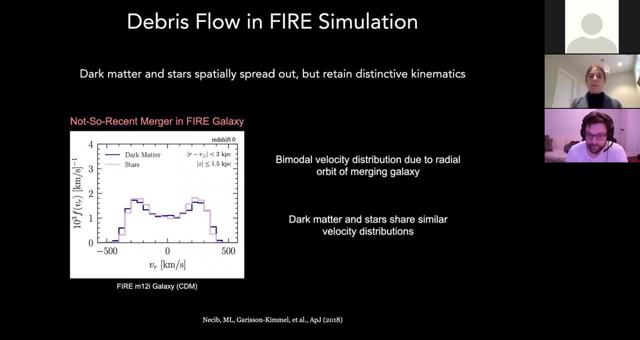 some interesting features left in it. So, for example, this is just looking at one of these not so recent mergers in the fire galaxy. Just plotting here the radial velocity of the material that's left behind by this merger and the dark matter is from that merger is shown in dark blue and the stellar material that's removed. 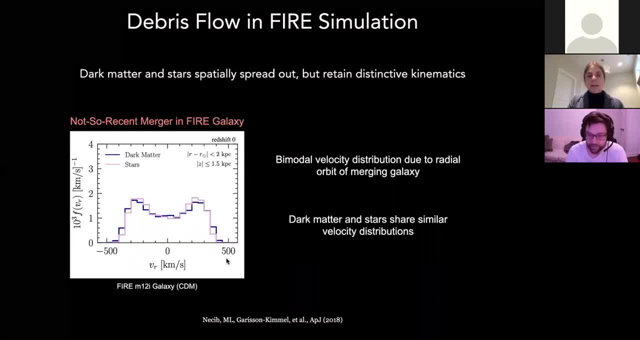 from that merger is shown in pink and you can see a couple things. One is that the velocity distribution has this kind of bimodality to it, which is an indication that the system hasn't equilibrated. So if it has equilibrated, you'd expect this to look more. 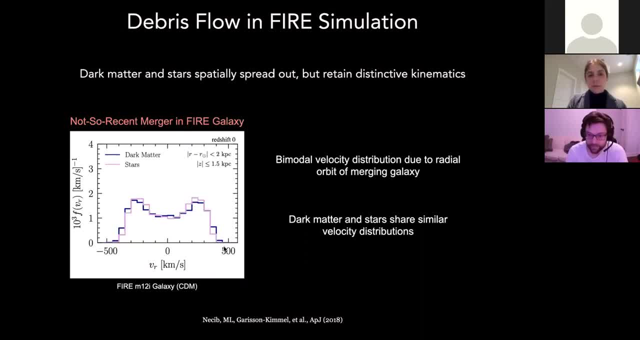 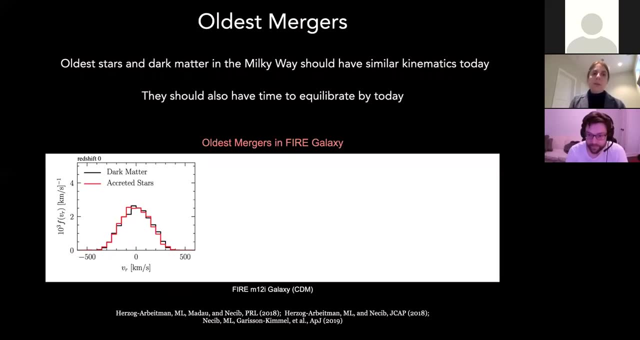 just like a simple Gaussian. The other thing that's kind of noteworthy about this is that you can see that both the stars and the dark matter. their velocity distributions seem to track each other quite, quite well, And the final stage of this is sort of the oldest mergers, the 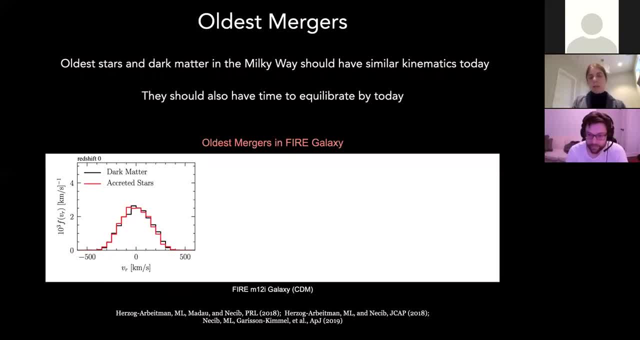 ones that came in a really long time ago. So they came in, they initially formed tidal streams as they were falling in. then that material was scattered and then it'd just start to fall in. Then it's a got all wound up, forming, you know, kind of a cloud of stuff left behind. So the position: 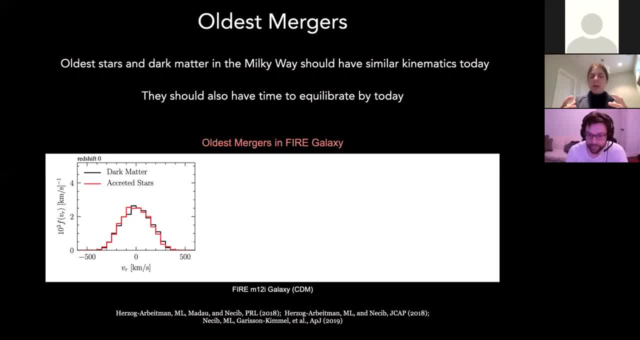 information gets washed out, but we still see the velocity behavior. But then if we let that evolve even further, what ultimately happens is that that material will just equilibrate with the Milky Way as a whole, And what we'll see today is really no interesting features in position, space or 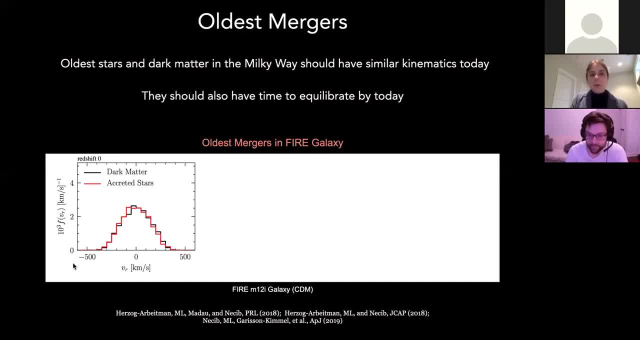 in velocity space. So here I'm showing material that's left behind by some of the oldest mergers in this fire simulation, Again starting here, just the radial velocity, Dark matter is in black and the stars from these mergers are shown in red. And because this material came in so early, 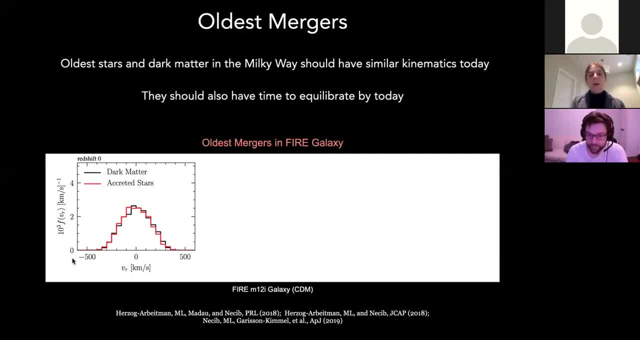 and has had a chance to equilibrate over time. the velocity distribution just looks Gaussian, So we've lost some of the interesting bimodal bimodality features that we saw in the previous slide. And then the other point to make is that 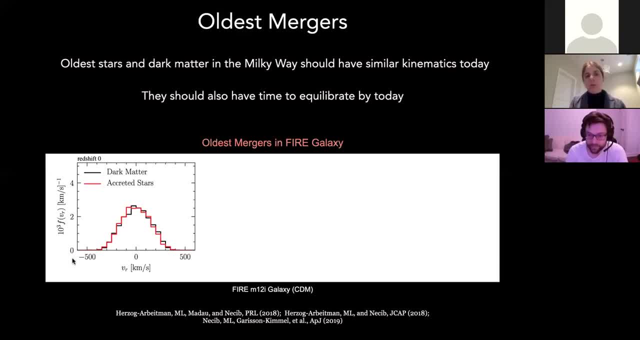 again we're seeing that the dark matter here the dark matter distribution, is tracing the distribution from the stars And while I'm here, I'm just showing a signal velocity coordinate. we see the same behavior even when we look at the other two velocity distributions. 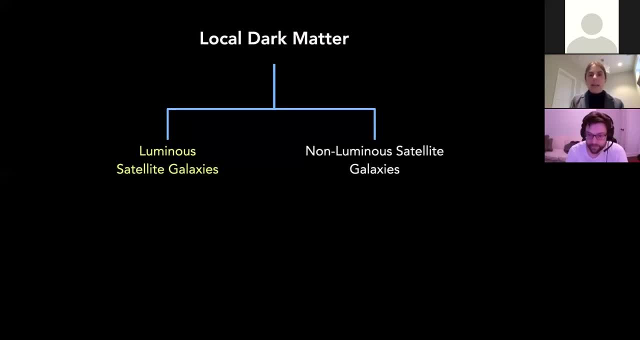 So let's take this all together and kind of talk about what our plan of attack is going to be. if what we want to do is create a map of the local dark matter, What we need to do is understand how that dark matter was dragged into our location in the 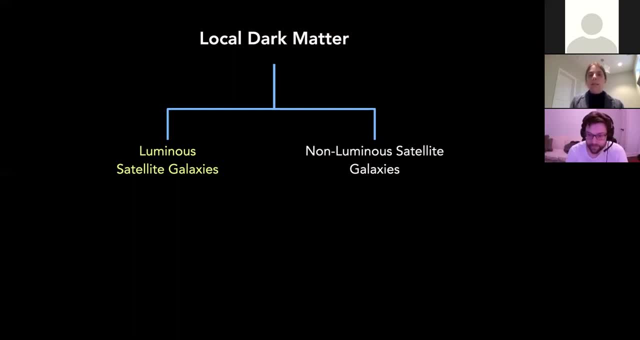 galaxy And the way in which it can be dragged in is through these mergers. Some of the mergers will have stars in them and we'll refer to those as luminous, so the luminous satellite galaxies that came in And some of the mergers, if the satellite galaxies are pretty small. 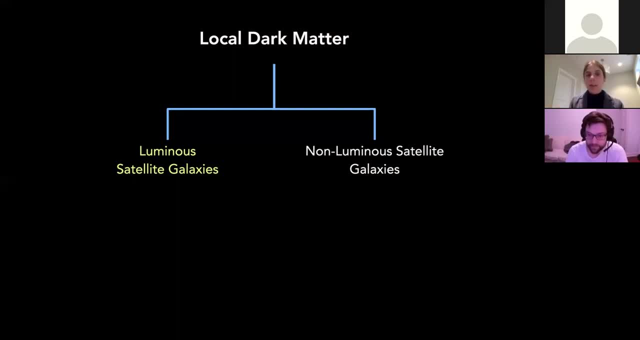 there will not be any stars in those galaxies. Now this case here, the non-luminous one, is particularly challenging, And at the moment what we've been decided to tackle is just the left. So we're starting by trying to understand what's been left behind by these luminous satellite galaxies. 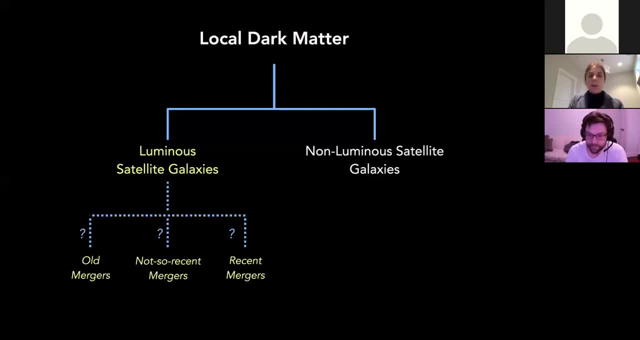 And then, under this category, then we want to know of the luminous satellite galaxies that have contributed material to our local area in the galaxy. how much came from the really old mergers, how much came from some of these not so recent mergers and how much came from you know. 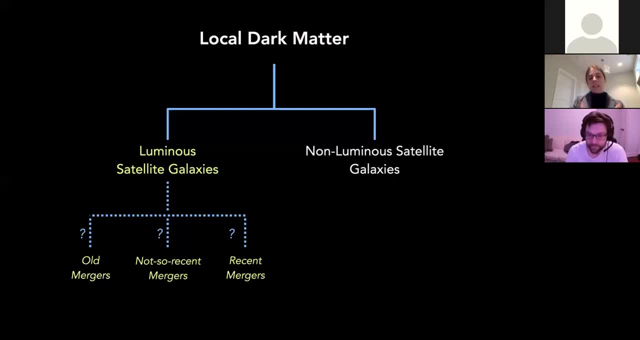 Anna Voelker, You know very recent mergers and the reason I divided these up into these three categories is that their position, the material left behind, would carry different position and velocity features, depending on Anna Voelker, Where, where we fall here. so this set of mergers would leave title streams. this set of mergers would leave pretty much just velocity, substructure, no position, interesting position, information, and this stuff here would leave material. that's all pretty much equilibrated by today. 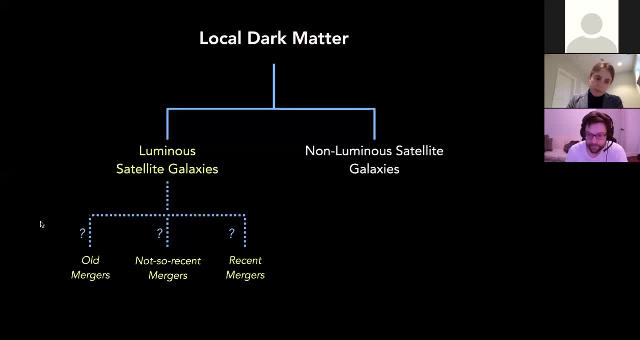 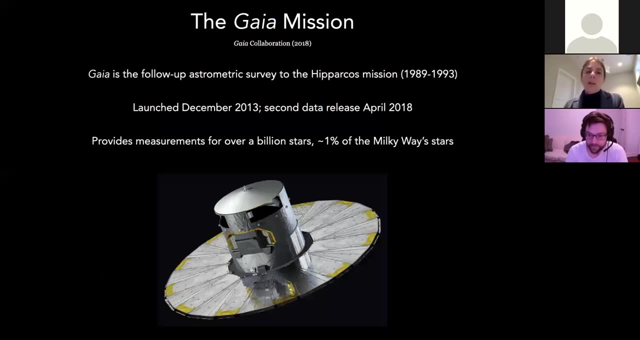 Anna Voelker. So for the rest of the talk, i'm going to show you how we've been filling in this part here at the diagram, Anna Voelker. And the reason we've been able to make progress in this direction is due to incredible data that's coming out of the Gaia satellite mission. 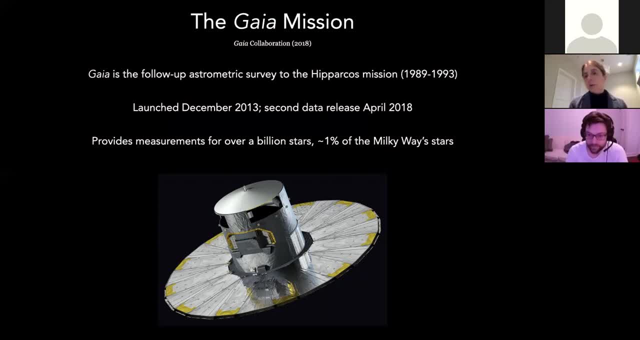 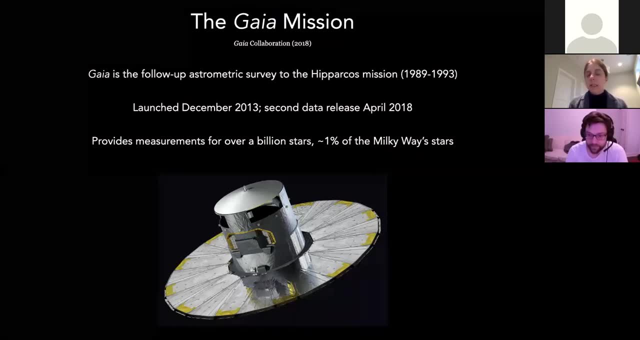 Anna Voelker. So that is the follow up astrometric survey to the parkos mission, which ran in the late 1980s- early 1990s, Anna Voelker. It was launched in December of 2013 and had its second data release in April. 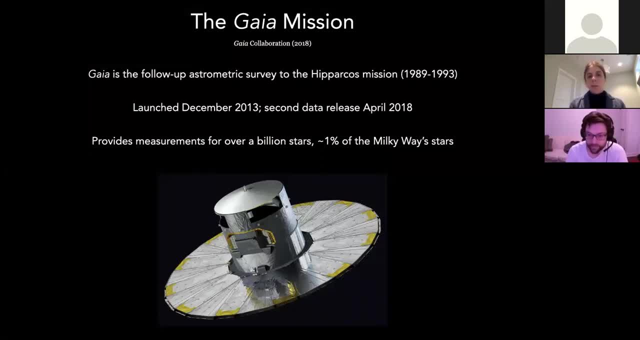 Anna Voelker In 2018, and it is providing measurements for over a billion stars in the galaxy, which is about 1% of all of the Milky Way stars. so this is a huge step forward in terms of the the amount and quality of data that we had. 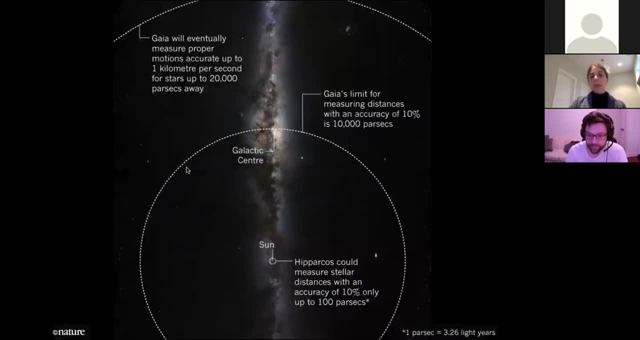 Anna Voelker Going back to her parkos and to kind of drive home that point, this is an image of the galaxy, the galactic disk, but rotated by 90 degrees, so it's vertical here, Anna Voelker. here's the sun. 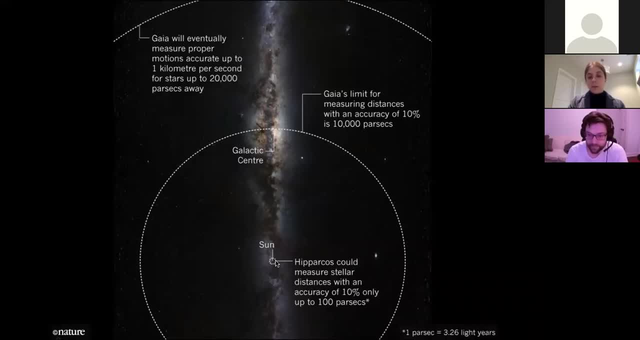 Anna Voelker, And this small little dash circle around it is the range where the parkos was able to get stellar distances to good accuracy, Anna Voelker, The comparable range for Gaia. so to sort of match that same level of accuracy goes out much, much further. so that's indicated here by this circle. 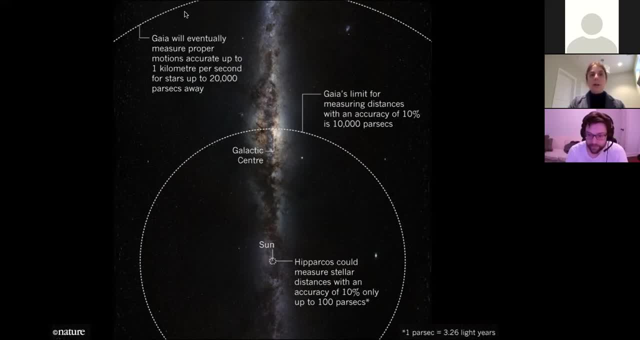 Anna Voelker And ultimately guy, is going to be able to do well at measuring motions accurate up to about a kilometer a second. Anna Voelker- All the way out here to this Anna Voelker circle, that's kind of getting cut off by the slide. 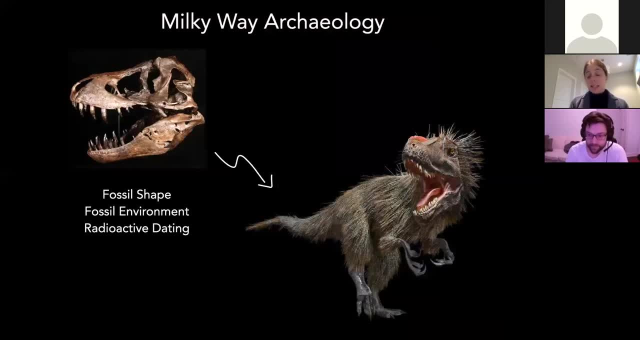 Anna Voelker. So what's the task? the task is to go into the guy data set and to try to find which stars they are actually came from some of these mergers. if we can identify those, then we can piece together some information from. 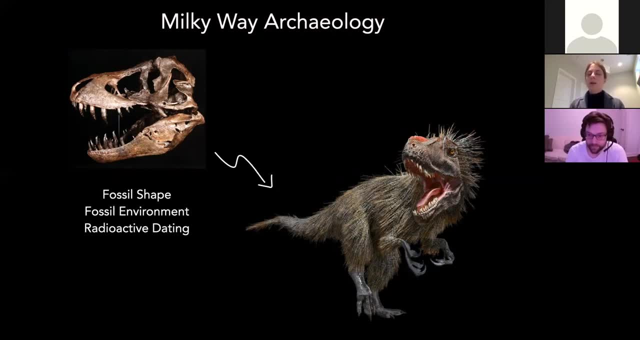 Anna Voelker, You know the properties of the mergers and then, based off of that, then also try to figure out where the dark matter from those mergers ended up. Anna Voelker, So this is a bit of a fossil hunt in the way that you know, same way that if you go on an archaeological dig and you find a fossil and you look at the shape of the fossil or its environment. 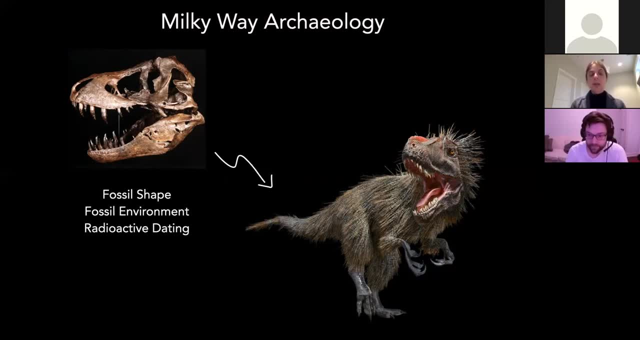 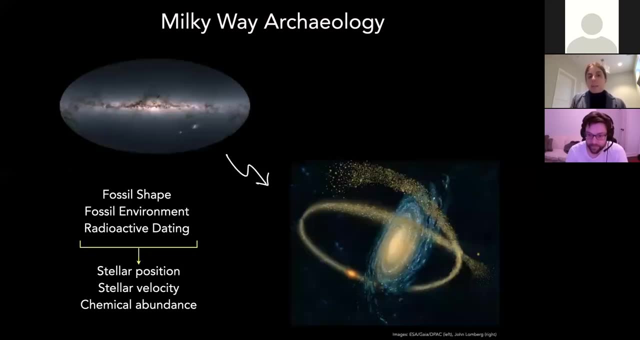 Anna Voelker, Maybe you do some radioactive dating. you're going to pull together all of that information and then try to infer something about the creature that that fossil came from. Anna Voelker, we're going to do something similar, but with the guy data. so what we have now is going to be, you know, information about the position of stars, their velocities, perhaps their chemical 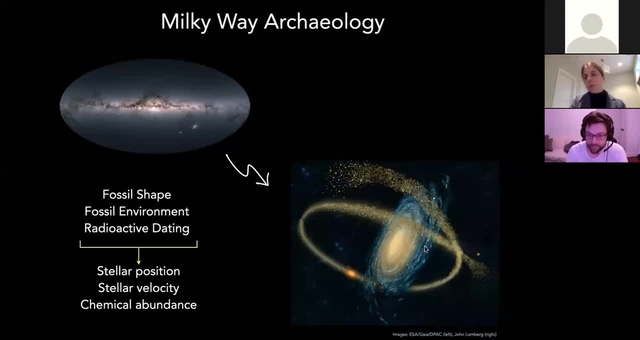 Anna Voelker And then, based off of that information, what we want to do is infer something about perhaps some merger that occurred a long, long time ago, Anna Voelker, That contributed to the growth of our galaxy. Anna Voelker, Now the top left panel here is actually the guy data, and if you can see that most of the like where the map here is brightest, is here, which is just the galactic disk. 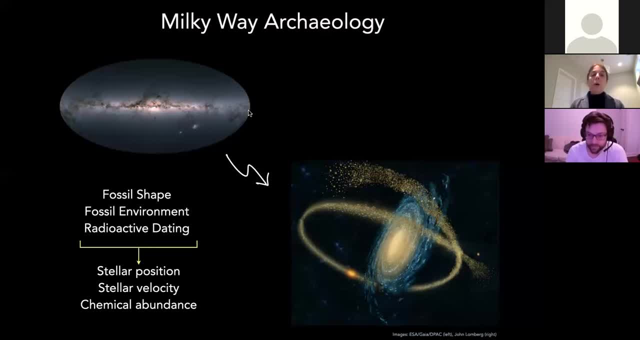 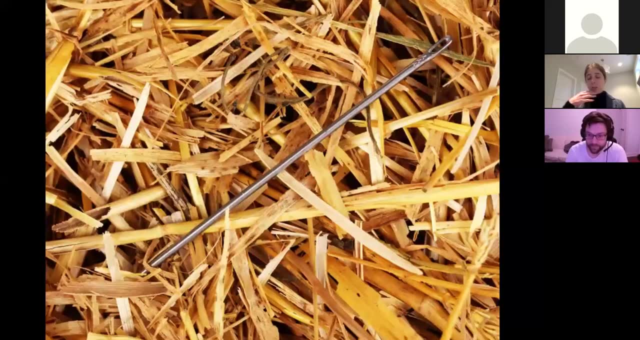 Anna Voelker. The vast majority of the stars that guy is observing are ones that were just Anna Voelker, born in our galaxy, so not ones that came from these mergers. so what we Anna Voelker. So this search is really when we are literally trying to find a needle in a haystack. we're trying to find very rare stars that could point us to some interesting historical note about our galaxy. 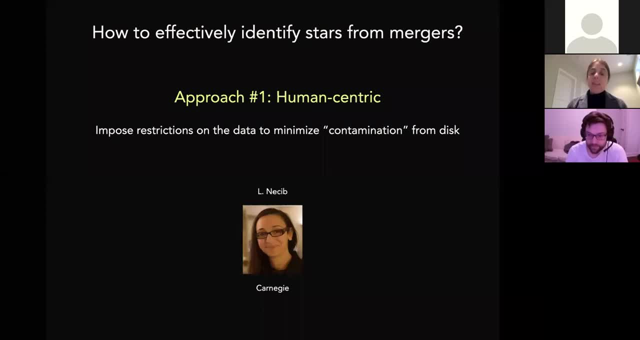 Anna Voelker. So we've taken a few approaches to doing this, and i'll present both of them. so i'm going to start off with the first one, which i'm going to call human centric, Anna Voelker, And this is in contrast to the second approach, which will be machine centric. so what we have on our hands is essentially a big data problem. 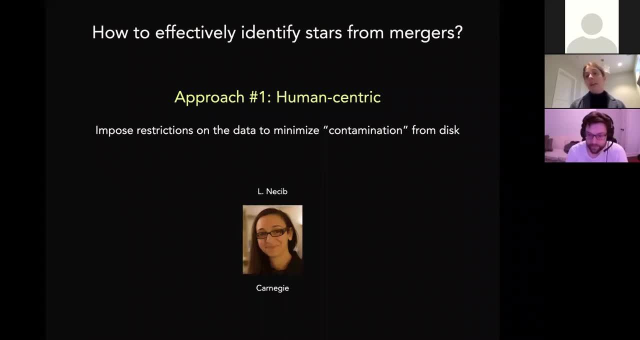 Anna Voelker guy, data is huge and we're trying to find rare events in this huge data set, Anna Voelker. If we want to do this, Anna Voelker In, so in approach one, what we're going to do is just impose restrictions on the data that can minimize the amount of contamination that you're getting from stars that we do not think are so. 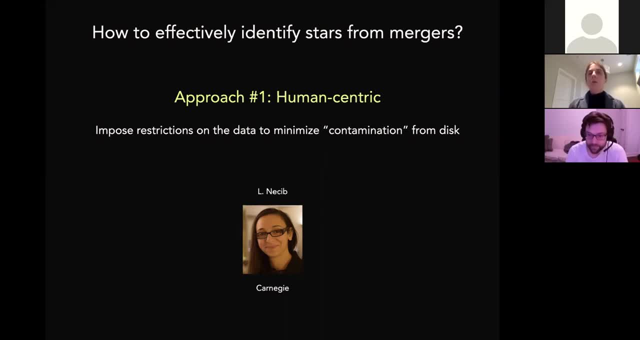 Anna Voelker, associated with these mergers, and so obviously you know, in order to get that that cleanest handle on this, we're going to be very conservative and place very tight restrictions to try to remove as much of these- let's call them- background- as possible. 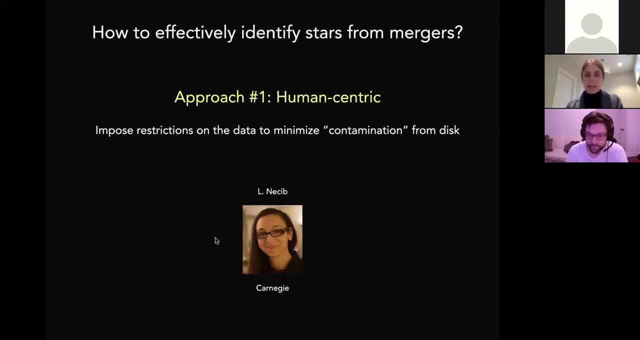 Anna Voelker, And the work that i'm going to talk about was led by postdoc Lena the seep, who is starting a new postdoc actually now at the Carnegie institute, Anna Voelker. um, so, as I mentioned in this approach, 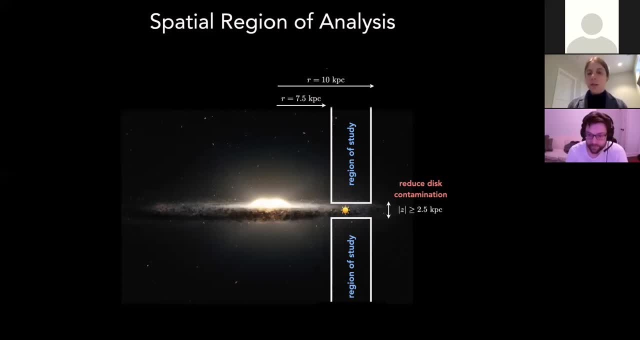 Anna Voelker, We're going to try to be very conservative. we want to try to pick out those rare stars that came from the mergers and we want to ignore as best as possible, stars that would be associated with the Milky Way's desk. 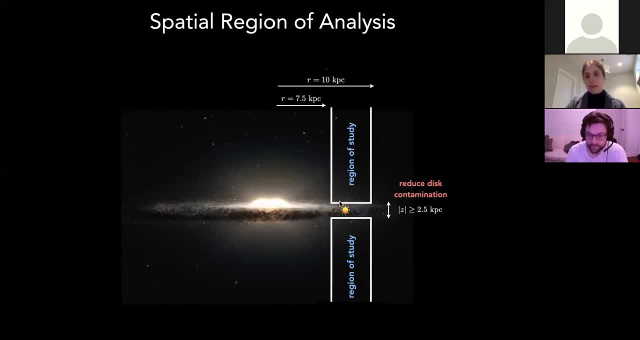 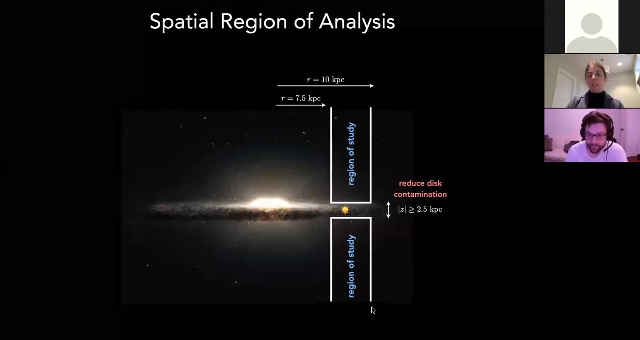 Anna Voelker. So to do this, we will specifically focus and place a cut on the spatial range that we're going to look at, Anna Voelker, And we're literally just cutting out everything. we're not even going to look anywhere inside the desk, we're just going to look in the region, this region here above the desk and below the desk. 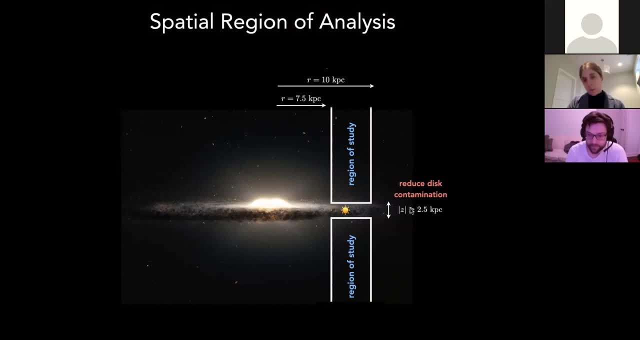 Anna Voelker- Again, this is an Anna Voelker, Very conservative- and just remove anything that we, this region here, where we know we're going to be dominated by stars that are not going to be associated with these mergers. 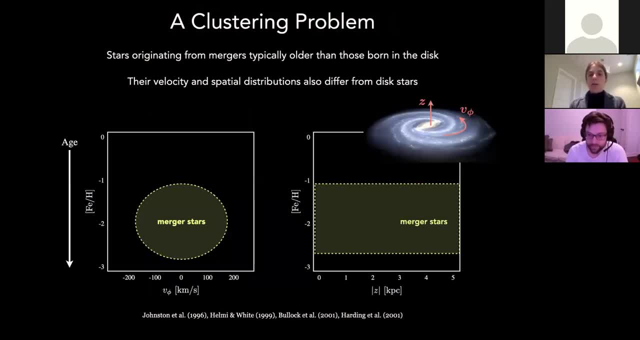 Anna Voelker, Even when we place these very strict cuts on spatial cuts, we're still going to get contamination from disk stars. so we'll need to employ employ additional discrimination criteria, Anna Voelker. So to do that, we can use. 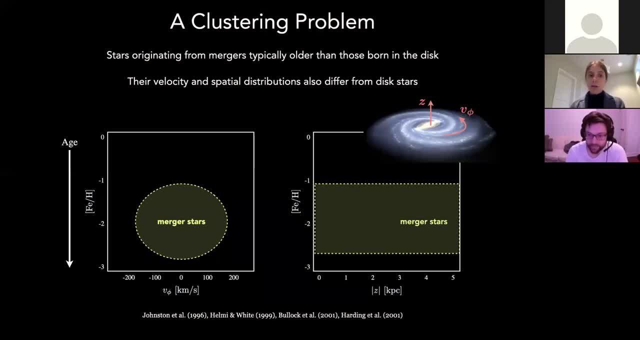 Anna Voelker. Information, for example, Anna Voelker, About the ages of those stars for which we use chemical abundance as a proxy, and also just their velocities. so for one example is if we just look at the velocities of stars in the desk. 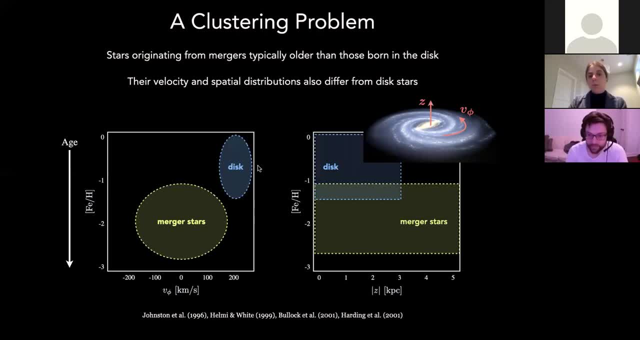 Anna Voelker. The stars that would be associated with the Milky Way's disk would be rotating, so we'd expect them to fall in this plot here in the upper right. they'd also be fairly young, so that would put them on the y axis of put them up here. 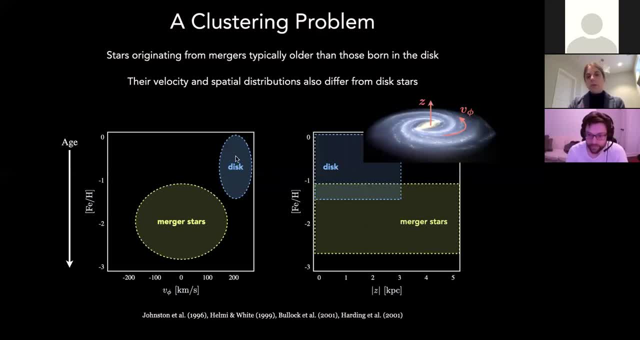 Anna Voelker, And in contrast, the stars that would be associated with these mergers would not necessarily be rotating with the desk, so we'd expect them to be Anna Voelker Here, and they would typically tend to be older than the disk stars, so a bit lower here on this wide plane. 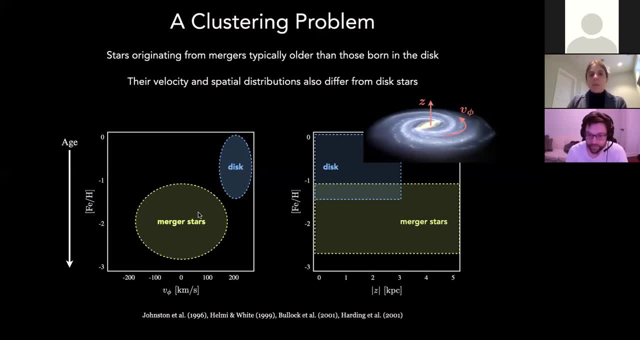 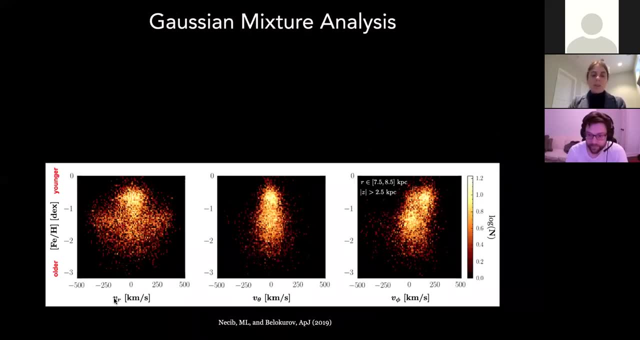 Anna Voelker. So we have here is actually a clustering problem, Anna Voelker. The data out of the box looks something like this, Anna Voelker. i'm showing here three different panels, Anna Voelker. The left panel has radio velocity, then this is angular velocity of data direction and in the five direction and the y axis is: 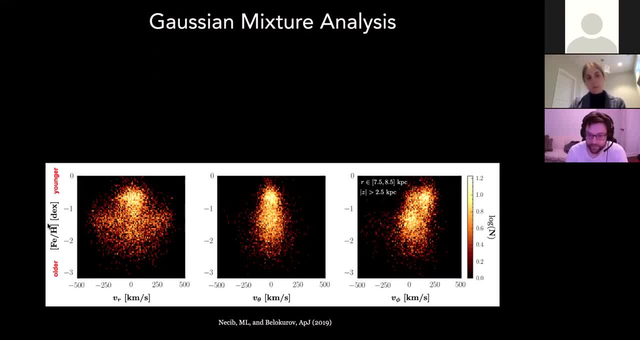 Anna Voelker, Chemical abundance. but if you're not familiar with that notation, you can think of this as a proxy for age. so anything at the top would be younger stars and at the bottom would be older stars, Anna Voelker. So out of the box, this is what the data looks like and you know the simple schematic I showed on the previous slide. 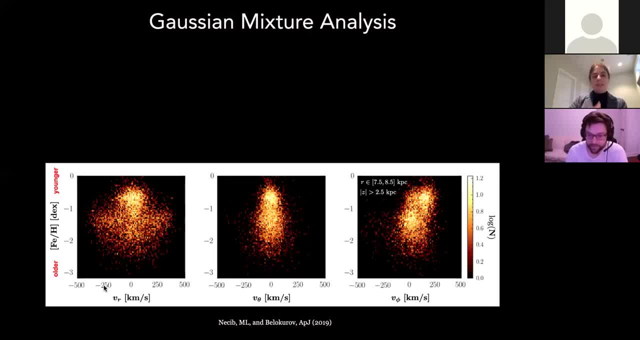 Anna Voelker. You know it may be a little bit hard, Anna Voelker, To see how that trend, you know, plies over to this case, because now it just looks like we have a big blob of stuff, Anna Voelker. And so what you want to do is to have apply a Gaussian mixture analysis to figure out how many different individual clusters of things are in this full data set. 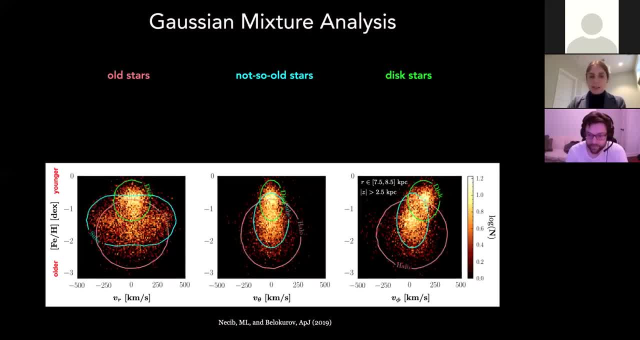 Anna Voelker. So here, when we do that Gaussian mixture analysis is the result of what we find. the circles- you're not ones i've drawn in by hand, Anna Voelker, Those are actually coming out from doing a full likelihood analysis. 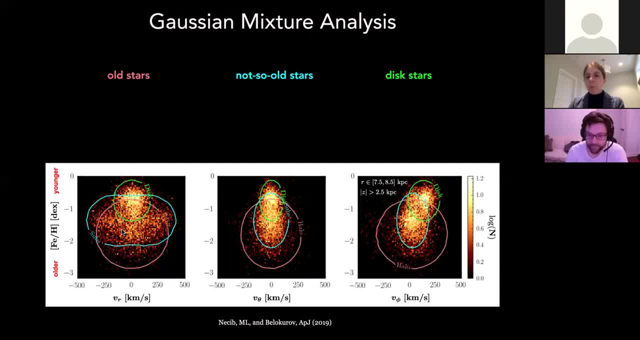 Anna Voelker, Where we finding that there is evidence for three separate populations in this total total data set. this literally just it's a. it's a Anna Voelker Standard kind of clustering problem. Anna Voelker, The three populations are associated with the following: so the green here would be the stars that are associated with the galactic disk, the, the red, 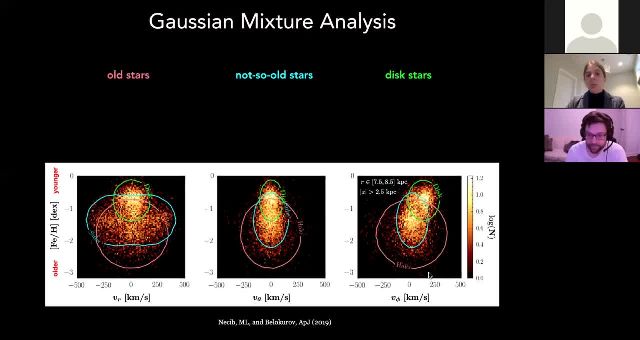 Anna Voelker, would be the ones that are associated with the oldest stars, so the ones that probably came in from the oldest mergers, Anna Voelker. And when you look at how these are, just in each of these different velocity components, their dispersion in each of the velocity directions is roughly the same, so it's pretty isotropic, we distributed, and velocity space 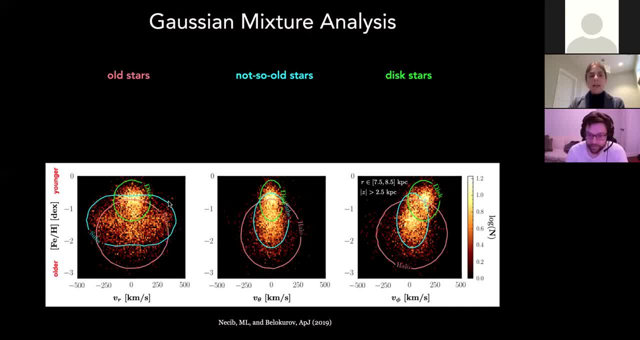 Anna Voelker. And then the blue cyan contour here is is intriguing primarily because it Anna Voelker, it's a bit more Anna Voelker The stars- you are older than the disk stars but younger than these really old ones here. and additionally, when you look at it in the radial velocity coordinate, it sort of squashed and and definitely looks like it has a radially biased. 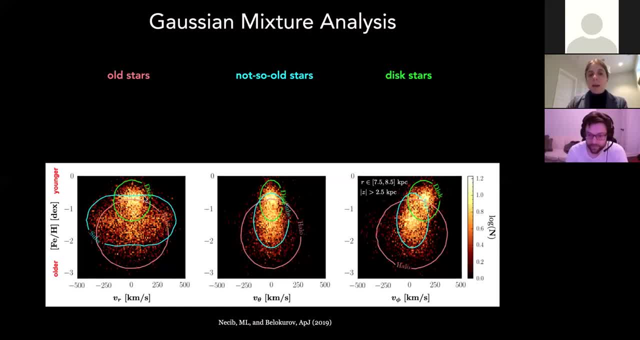 Anna Voelker. And so, in terms of our understanding of how these could map onto the dark matter, Anna Voelker, The things that are interest, potential interest, are the pink here, which, if this is associated with the oldest mergers in our galaxy. 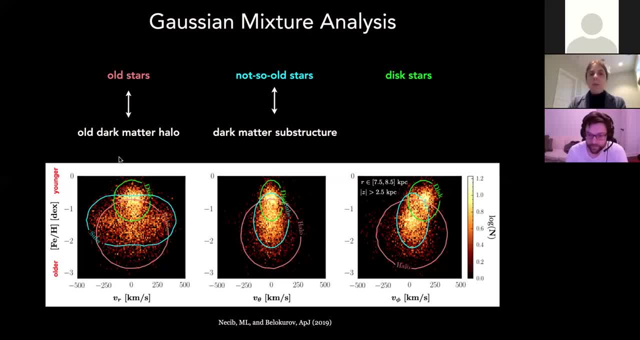 Anna Voelker. That would be telling us something about, Anna Voelker, The component of dark matter that's coming from these really old mergers. and then this cyan component here which, if it's coming from a not so recent merger, might be telling us something about a component of dark matter that's in some structure. 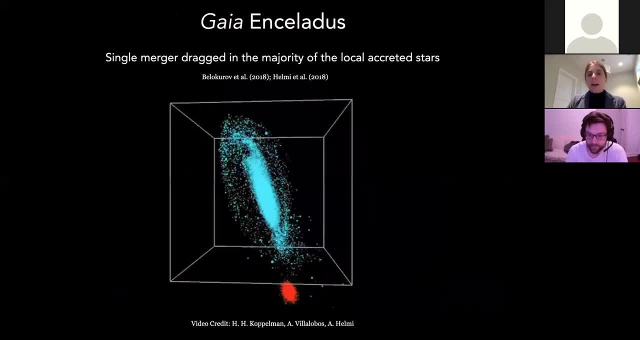 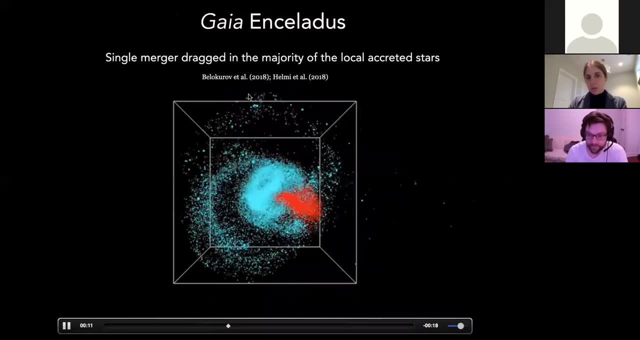 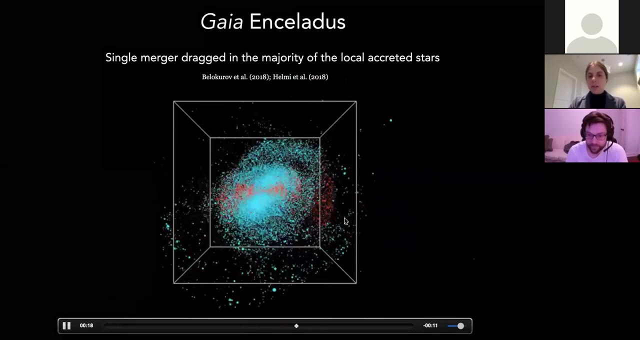 Anna Voelker. So that not so recent merger actually has a name. it's called Gaia and Saladas and it was first Anna Voelker, posited by Anna Voelker, The silly Bella crows group- and I mean a home use group- pretty soon after the second guy data release came out. the movie that i'm showing here is: 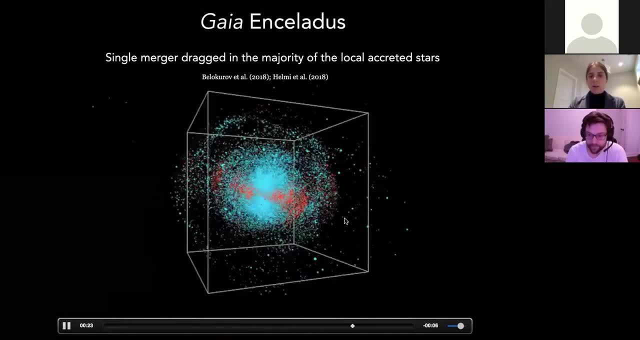 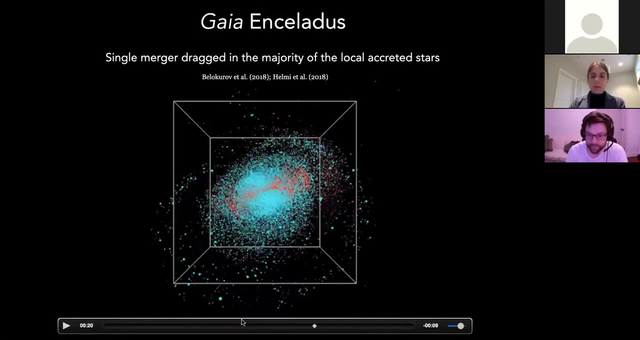 Anna Voelker, An image is actually just showing me the fallen of a galaxy and a lot of us and what it would look like ultimately once it's disrupted, so I could get that movie going again, Anna Voelker. So the red comp here would be, and so on. it says it's just beginning to fall in. 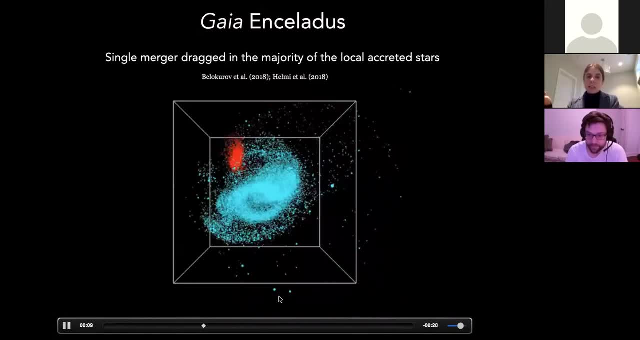 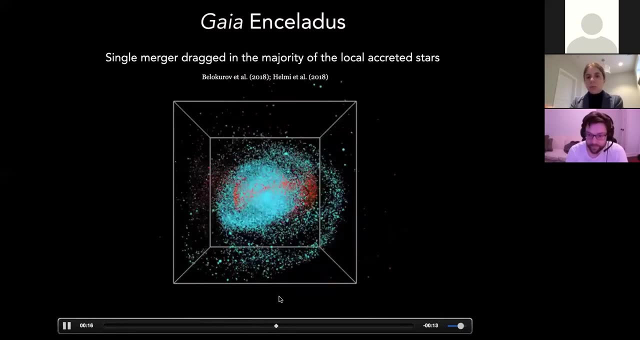 Anna Voelker should start going into Anna Voelker. There we go, and now it's going to be tidally disrupted as it continues several passes through the Milky Way, and then at the end you can sort of see where all of its stellar material gets left behind. 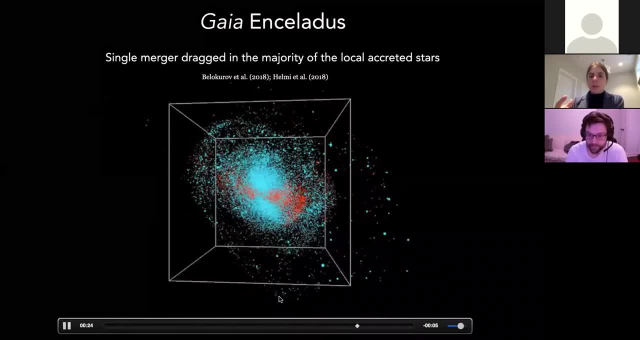 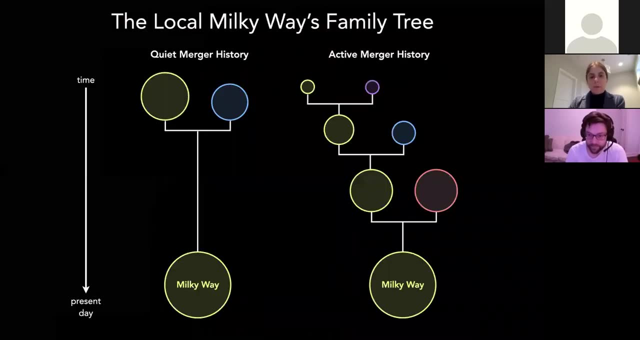 Anna Voelker, And it's concentrated in the inner part of the galaxies. that's one of the Anna Voelker key features of this particular murder, Anna Voelker. So, coming back to what this tells us about our family tree, 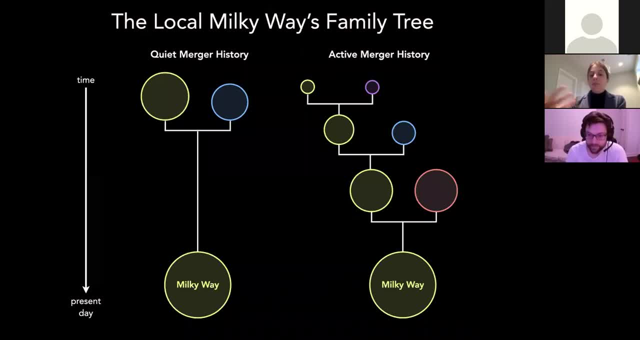 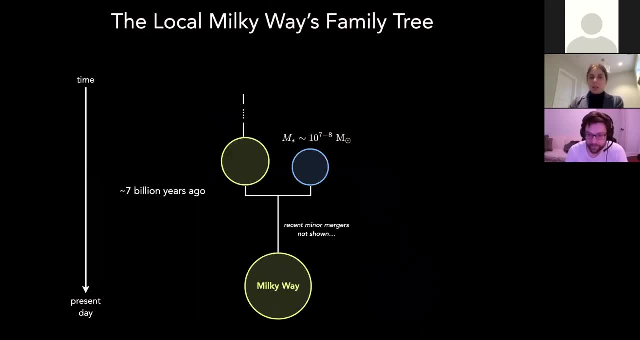 Anna Voelker. This is an important Anna Voelker piece of information in terms of kind of reducing down our number of possibilities. what it tells us is that about 7 billion years ago, there was a fairly significant merger that came in, and at that time this guy- and so a lot of us- was probably about 10 to the 710 to the eight times the mass of the sun. 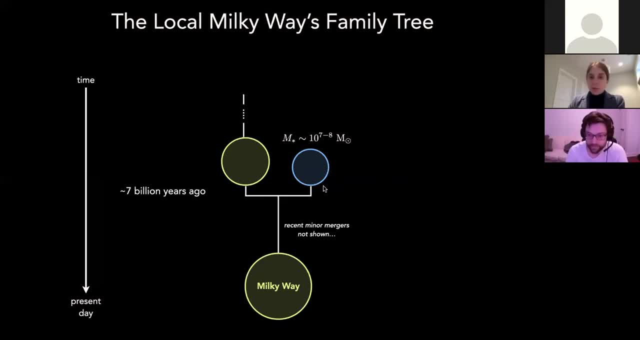 Anna Voelker. So it pins down one of our oldest neighbors- not neighbors- Anna Voelker, Relatives. so pins down one of our oldest relatives, Anna Voelker, um. Anna Voelker And also indicates: because this occurred about 7 billion years ago means it's not too soon, but also not too early. so it's precisely in a regime where we would 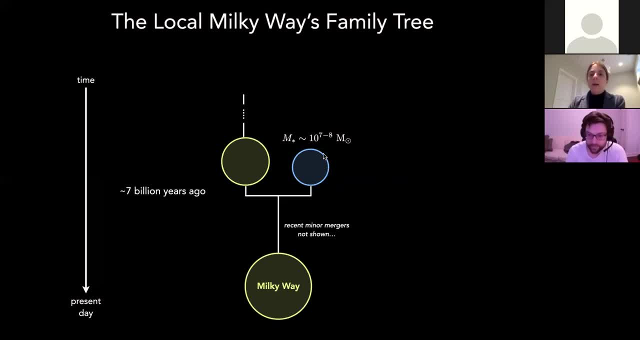 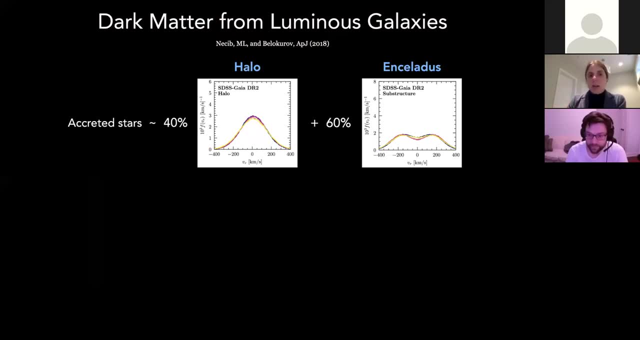 Anna Voelker, Where we know from simulations that the dark matter that's left behind would not have had enough time to to come into equilibrium. Anna Voelker, So if we take all of this together, what we extrapolate to the dark matter, and I 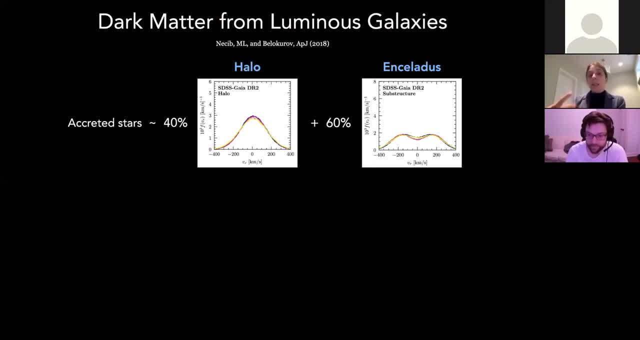 Anna Voelker will just give you kind of the final result here and I don't have time to kind of go into detail in terms of the Anna Voelker Full steps that we take in doing this extrapolation. but what we find is from the stellar component that about 40% of the stars 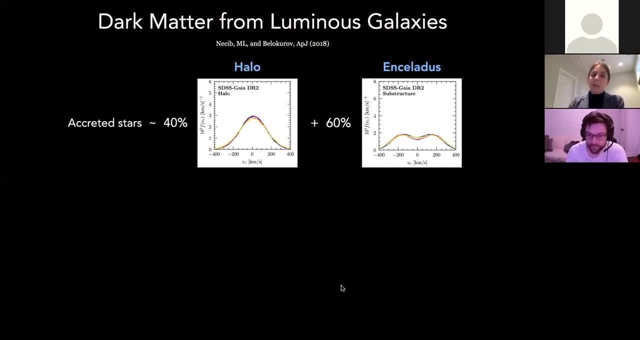 Anna Voelker, Near near us in the Milky Way, are in, came in from these really old mergers and about 60% came in from this new relative and a lot of us and when we do the appropriate extrapolation to the dark matter that would have come in. 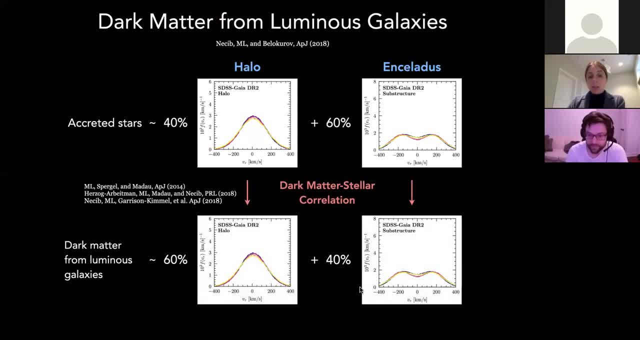 Anna Voelker. That would have come in, Anna Voelker, From the same sources. what we find is about 60% of the dark matter would have come from these very old mergers and about 40% would have come from from Enceladus. 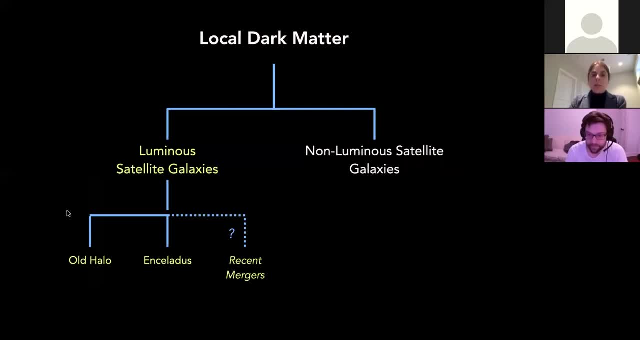 Anna Voelker. So that already like starts filling in some parts of this diagram. here on the left, Anna Voelker, we're seeing evidence for material that came in very early on, and then also material that came in a bit more recently from this new merger. that's called Enceladus. 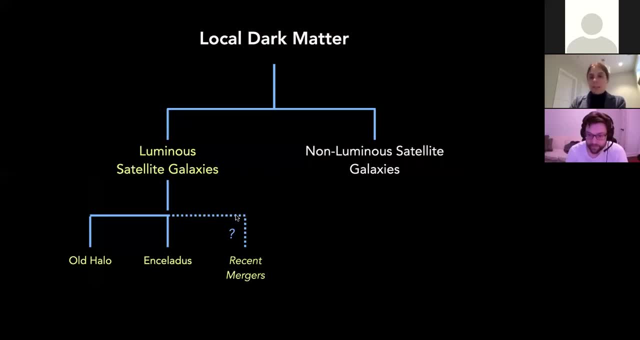 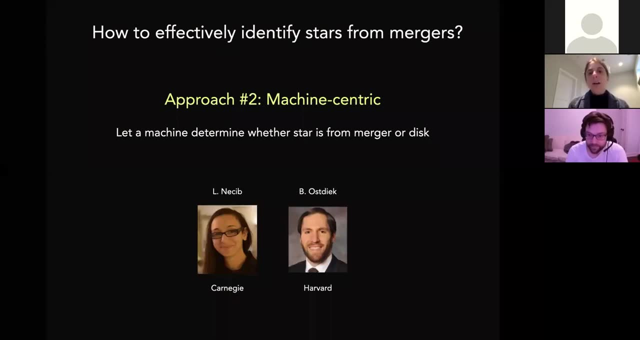 Anna Voelker, And what we want to know is: is there anything that came in even more recently than that? and that takes us to the second approach and the last thing that I want to highlight: um, so this is taking a machine centric approach. 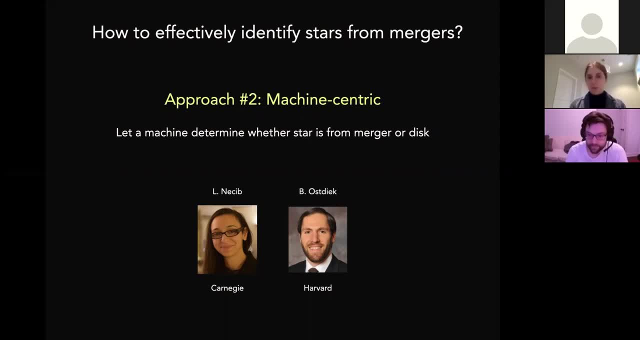 Anna Voelker. Now, what we want to do is let a machine determine whether or not a star is coming from a merger or whether or not it was born in the disk. Anna Voelker, And this part of the work is led by Alina Nassib and also Brian Ostiak, who's a postdoc at Harvard. 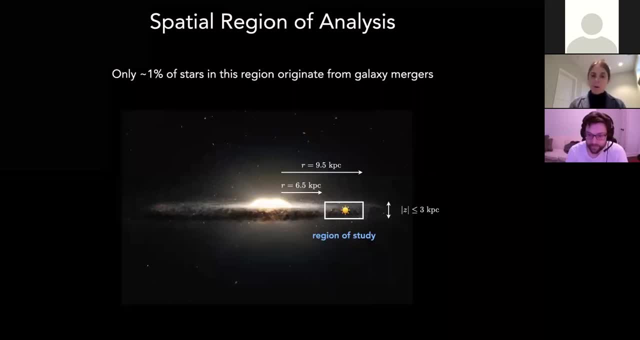 Anna Voelker. So before we were extremely conservative in the cuts that we placed and we were specifically trying to avoid looking at anywhere close inside this disk because we knew that we would be largely contaminated by disk stars in this regime and indeed only about 1% of the stars here originate from 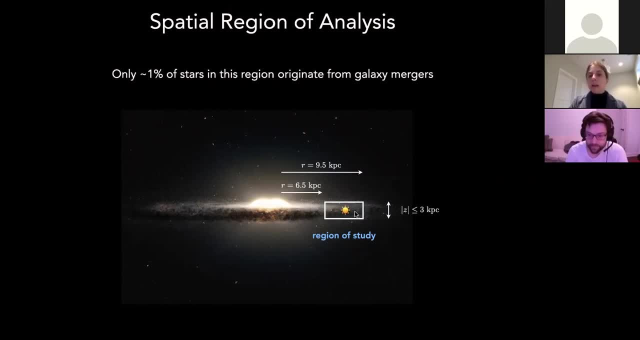 Anna Voelker From galaxy mergers. So we're really really looking for very rare events here, Anna Voelker. Now that we're going to let a machine, Anna Voelker, We're going to throw this problem to a machine. 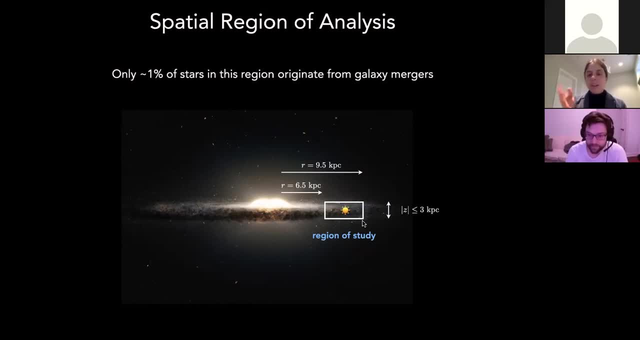 Anna Voelker. We decided to just tackle this, go right to where the hard problem was and to see if we can have the machine actually distinguish of the stars in this regime, which ones are disk stars and which ones came from the mergers. 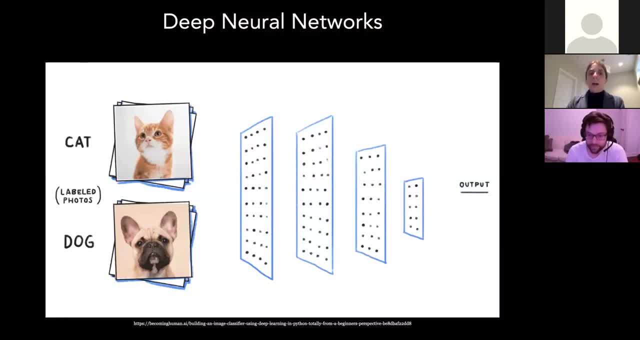 Anna Voelker. So to do this we used neural networks. Essentially this is a classification problem, So kind of a characteristic, or the Anna Voelker Very common example for classification networks, Anna Voelker, Is you train on a picture of cat and pictures of dogs and the network learns how to distinguish these two. So it starts off with these labeled photos and then 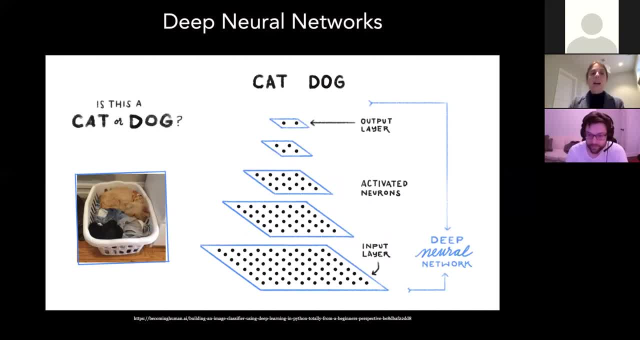 Anna Voelker, You apply your network to some other photo that you happen to have and the network, given what it's learned from the labels training set, can then distinguish and identify whether or not this new photo here is a cat or a dog. 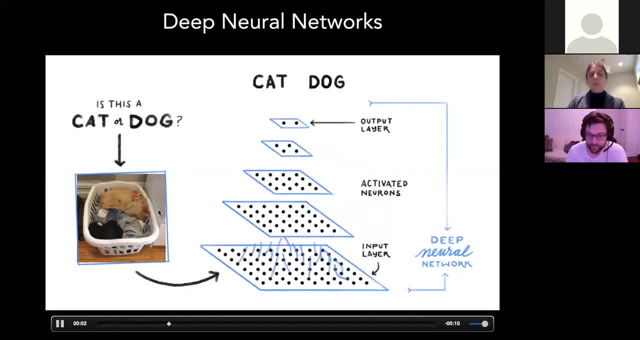 Anna Voelker. So what we want to do is going to be a similar, except instead of Anna Voelker Working with pictures of cats or dogs, We want to instead work with simulation images or simulation information of stars, where the stars are labeled as either being born in the Milky Way or born from inside- one of these mergers that got dragged in. 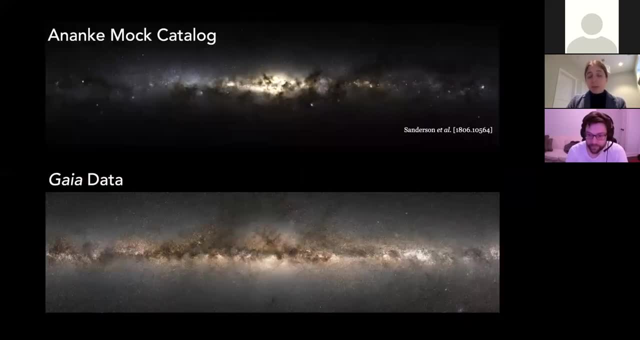 Anna Voelker. If you know, the only reason that we have any shot at having this work is because the quality of the simulations have gotten really good, Anna Voelker, Recently. on this slide I'm showing- on the top, Anna Voelker, Is a mock catalog of of the Milky Way galaxy and on the bottom is the actual Gaia data. 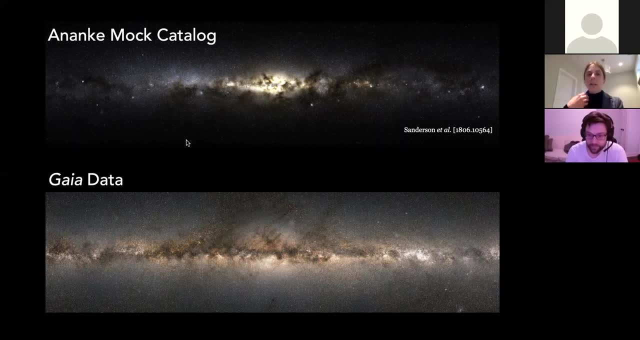 Anna Voelker. What's going into this mock catalog is all the information about the hydrodynamics of how our system is, how our galaxy is built up. so information on the gas, the stars. there's feedback that's fed into dark matters also there. 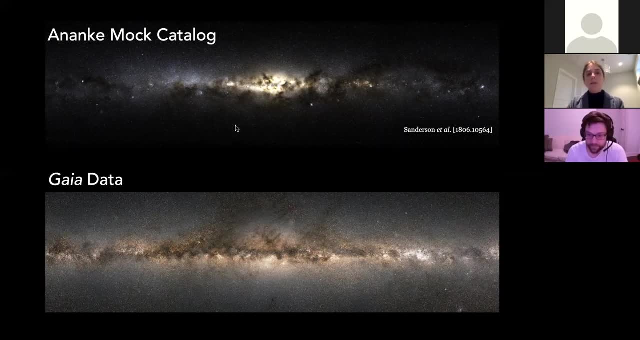 Anna Voelker, And it's quite remarkable that many of the features in this mock catalog reproduce what we're seeing in the Gaia data. Anna Voelker, It's not perfect, but considering the fact that perhaps decade- you know, a decade or so ago- the simulations couldn't even reproduce stable disks, It's quite remarkable The level of like, how far and how sophisticated the simulations themselves have gotten. 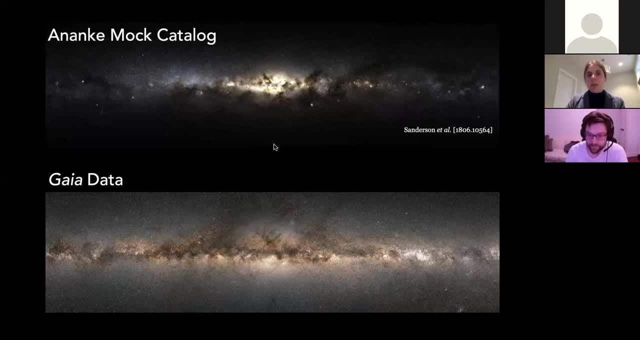 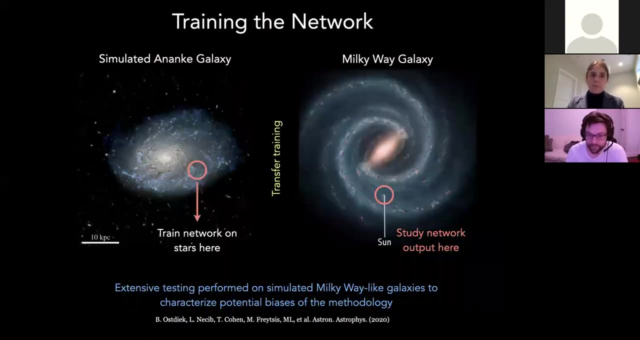 Anna Voelker. So what are we're going to do, then, is to use these simulations to train on them. These are essentially going to be our label data sets, and then we're going to apply the results to the Gaia data, Anna Voelker, And so I won't go into the nitty gritty details. for all of this, We did really a huge amount of testing to make sure that this worked, And I could probably give a whole- you know, another whole hour seminar on that, but very, very briefly, 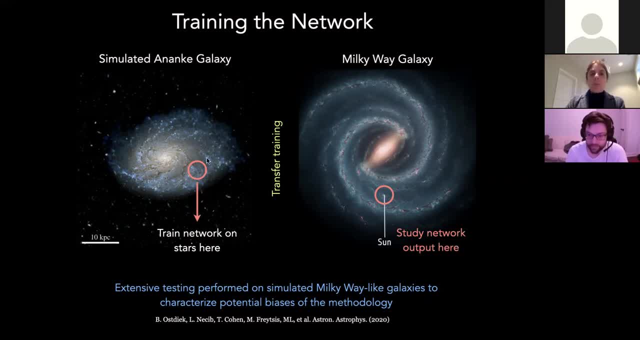 Anna Voelker. What we start with are the simulated galaxies. we train on stars there because, because it's a simulation, We actually know the origin of those stars, So that's our label data set. Then we apply what's called transfer training, so we 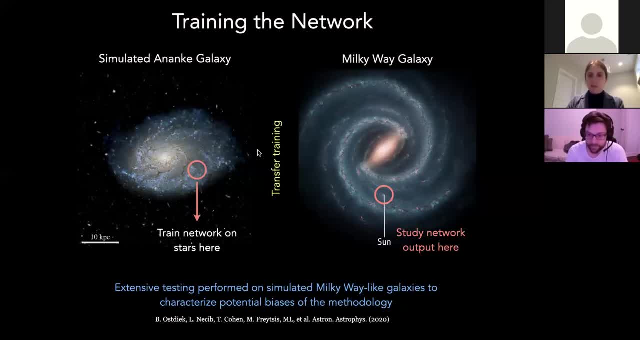 Anna Voelker, Retrain the last layer of the network using a very small subset of actual real data that we think has a high, high purity identification of disk versus Anna Voelker Halo stars. and then we apply, ultimately apply the network to the actual Gaia data. 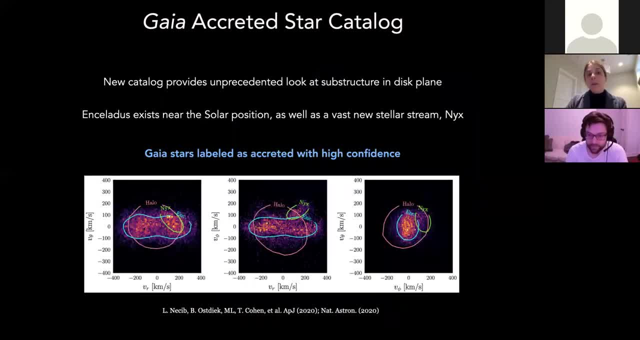 Anna Voelker. So, after applying this process, What we can do is we can actually build a new catalog, Anna Voelker, Of the stars that the network predicts are coming from mergers. And what I'm showing here in the bottom is a is are the velocities of all of the stars that network has predicted to be born outside of our galaxy. 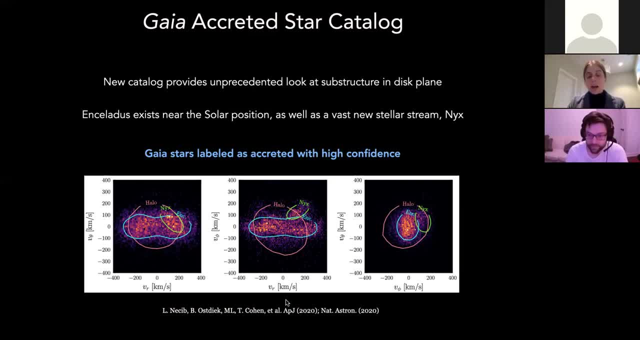 Anna Voelker. And again, then, we have to apply a clustering algorithm to this to identify the individual pieces that are distinctive in this three dimensional space, And what we find are the following. So the pink here, Anna Voelker, Is corresponds to the stars that came in from the earliest mergers. the blue, 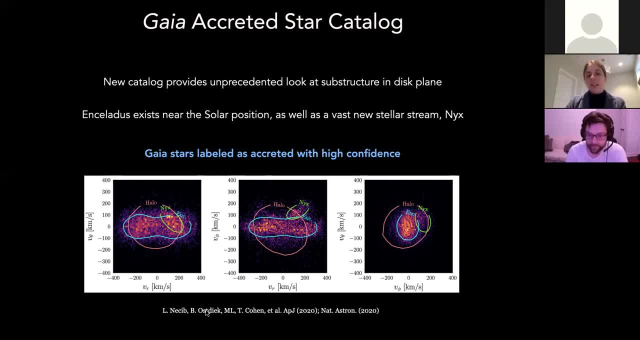 Anna Voelker Cyan corresponds to the stars that came in from our new relative, Enceladus. So this is actually interesting because it shows us that Enceladus also dumped a bunch of stuff right close to where the sun is, which is important for for underlining the fact that that dark matter from Enceladus will be relevant for any kind of terrestrial search. 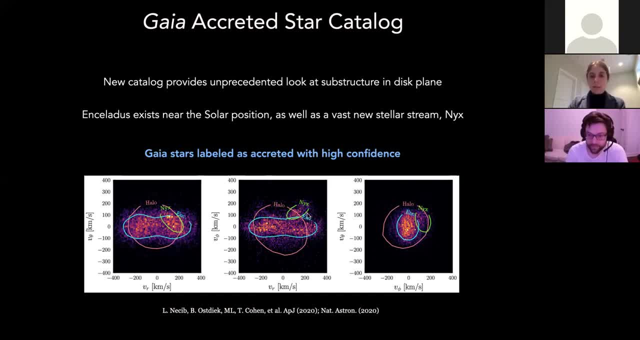 Anna Voelker. And then, in addition, we find a new structure, which is shown here in green, And this we've called Nix, after the Greek goddess of the night. So that was the image that I actually started off my talk with. 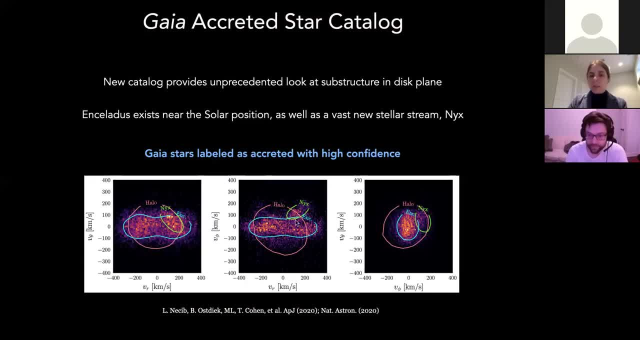 Anna Voelker And the stars that the clustering algorithm finds is being associated with this next structure. are Anna Voelker, Really? quite their. their kinematics are really interesting. So they have a very high radio velocity, So almost 200 kilometers a second and they are. 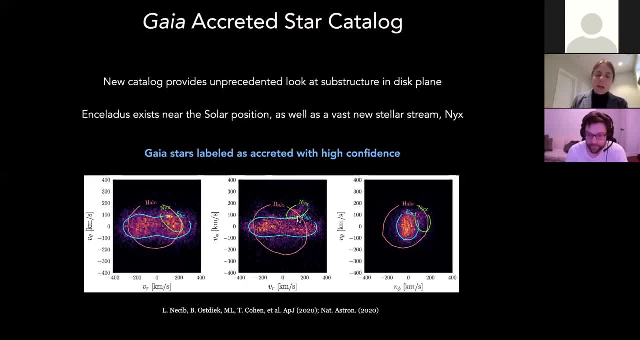 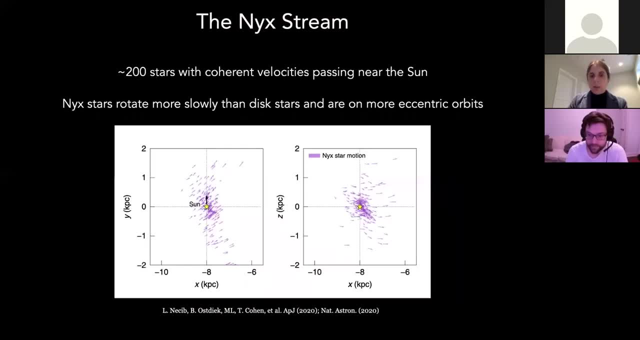 Anna Voelker, Rotating close to, but not exactly with the speed of the sun around the center of the galaxy, The. their orbits are very eccentric, Anna Voelker. If you want a way of kind of visualize this a bit better, This is looking at all of those stars in that stream. 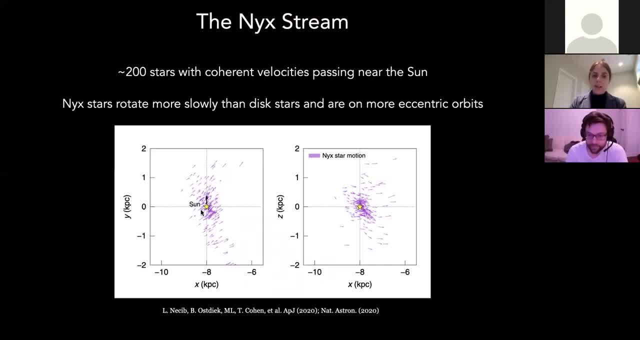 Anna Voelker In a top down view of the galactic disc. so x and y here. Here's the sun moving up in this coordinate frame and each little purple arrow here is a star that is associated with Nix Anna Voelker, And you can see by eye that the 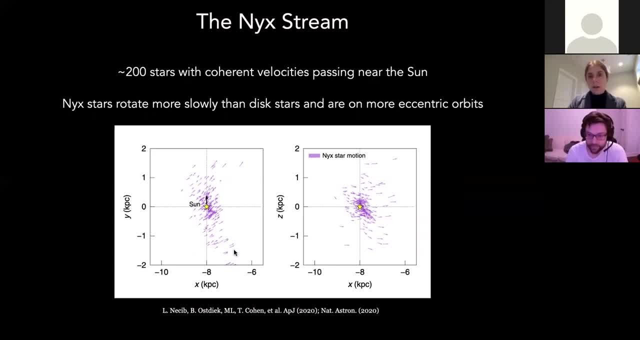 Anna Voelker, The the motion of the stars is very coherent and it also that their orbits are more eccentric than what we expect from from the sun, Anna Voelker, So this is an intriguing structure that we find and it's stream like, which suggests that if it did come from a merger, that that merger would have probably occurred fairly recently. 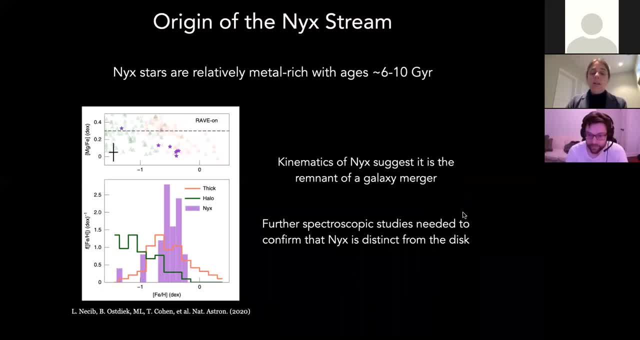 Anna Voelker And Anna Voelker, The. our next step is to confirm the origin of the stars. Anna Voelker, There's a variety of tools that we can use to help clarify whether or not these stars actually came from a galactic merger. we can look, for example, at the stars chemical abundances. we can try to infer something about their ages. 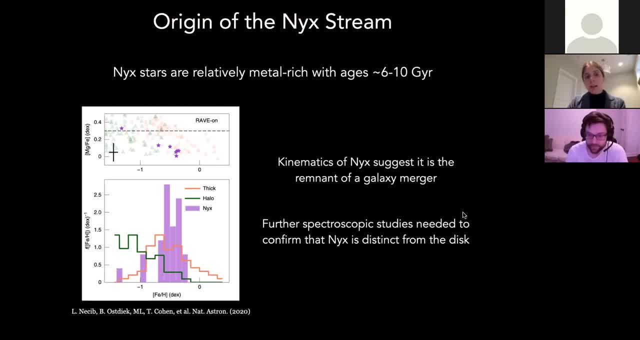 Anna Voelker. Unfortunately, even though we see about 200 of these stars that have this Anna Voelker, That are in this stream, Very few of them have associated chemical abundances- Anna Voelker Of the very few. So we only have about a handful that we see the chemical abundances for. the abundances look dislike but would not necessarily be inconsistent with coming from a merger as well. 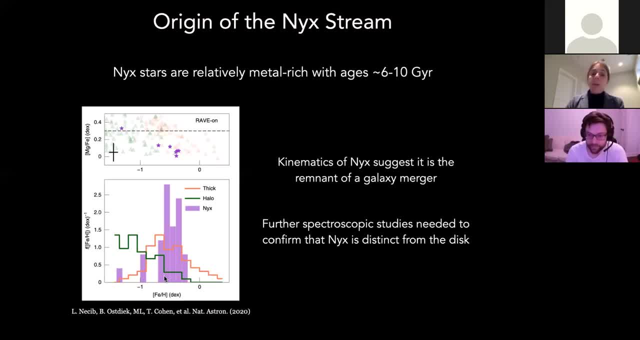 Anna Voelker. So really to be able to completely and robustly break this degeneracy between these two possible explanations, What we need is dedicated follow up spectroscopy of the stars, and that work is actually currently underway. So there is a team from Caltech that 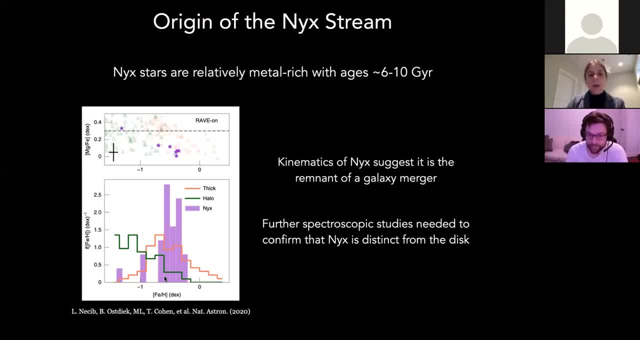 Anna Voelker Has run a bunch of these Anna Voelker Observations over the summer and is currently analyzing these results, and their study should be able to shed some light as to whether or not the stars that we're identifying and next originated from the desk or truly from one of these galactic mergers. 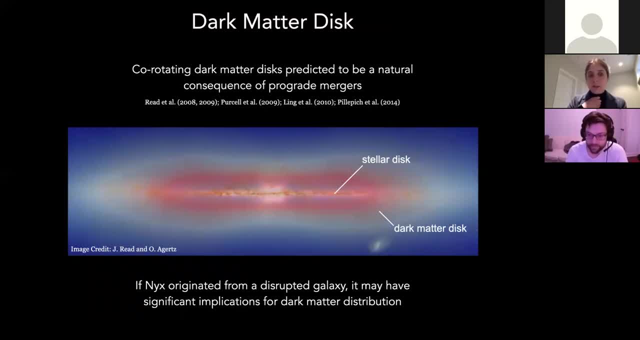 Anna Voelker. Now, as a dark matter physicists, The reason that I care about this next stream is that the kind of if it did originate from a galactic merger on, what it would have left behind is a dark matter desk, Anna Voelker. So we ordinarily just think of the dark matter in our galaxy is being distributed in this massive halo in order to have a stream that's aligned with our plane, similar to what we're seeing with next. that galaxy that would have created next would have also created. 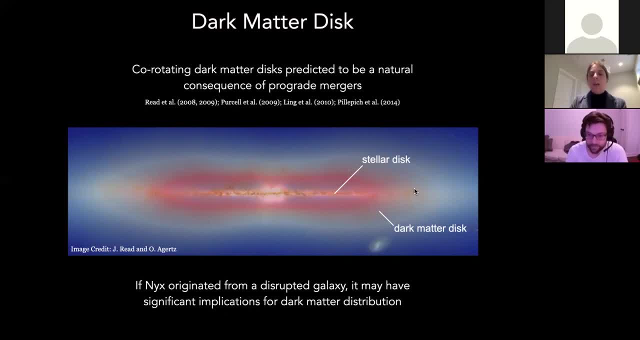 Anna Voelker- Essentially a large puffy dark matter desk that's surrounding our visible desk and rotating with it, Anna Voelker. So in this new picture we would have a dark matter Anna Voelker And then inside of it We'd also have a puffy little dark matter desk that's rotating around the center of the galaxy. 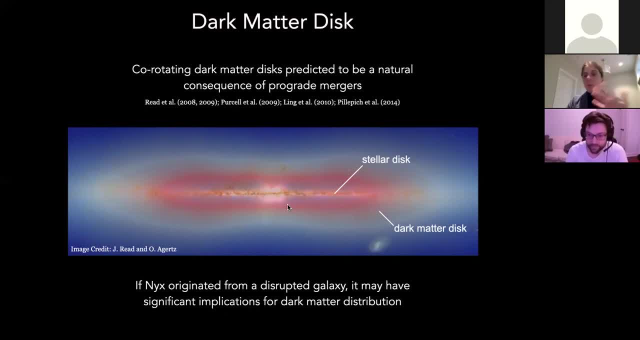 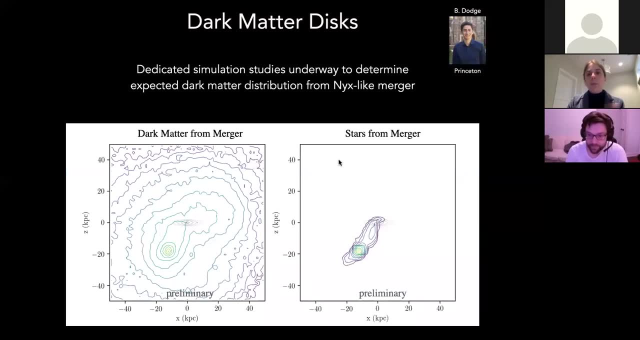 Anna Voelker To better understand exactly what the properties of this dark matter desk would be, how it forms, how it kind of correlates with what we're seeing from the next stars. Anna Voelker, We are actually running some dedicated simulations. This is work that's being led by an undergrad here at Princeton, Ben Dodge. 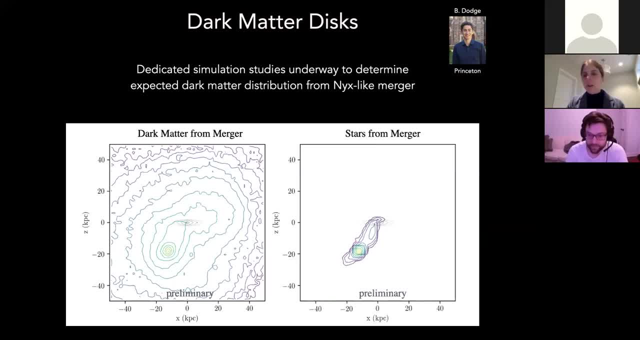 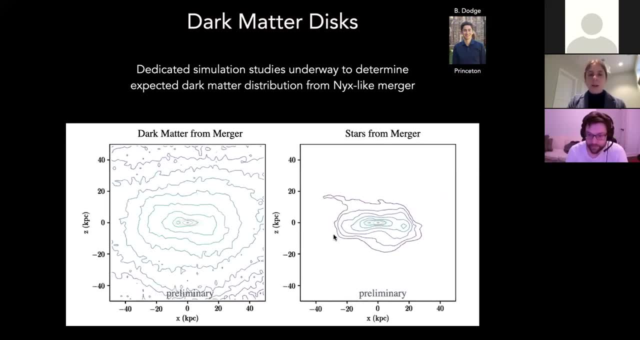 Anna Voelker, And so he's running simulations that track the Anna Voelker Infall of galaxies, small satellite galaxies, as they get torn apart and then form Anna Voelker Structures that look like Nix, And then we can also from the simulation see where the dark matter ends up, and the dark matter always ends up looking like this puffy rotating dark matter desk. 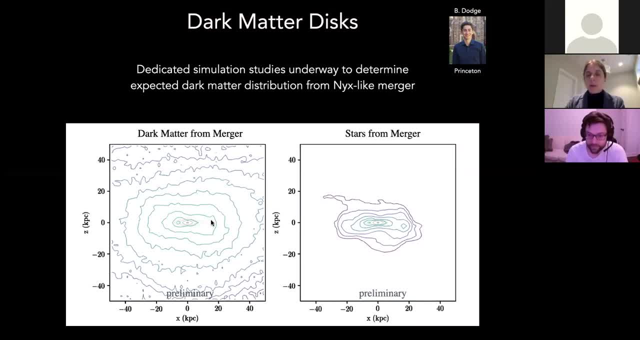 Anna Voelker. So I think you know, with the follow up spectroscopy, Anna Voelker, We'll really get a good understanding as to whether or not Anna Voelker, Nix is originating from these galaxies, Anna Voelker, And if it is, then we'll really need to understand in detail from simulations like this exactly what the properties of that rotating dark matter disk would be and what the implications would be for any terrestrial dark matter search. 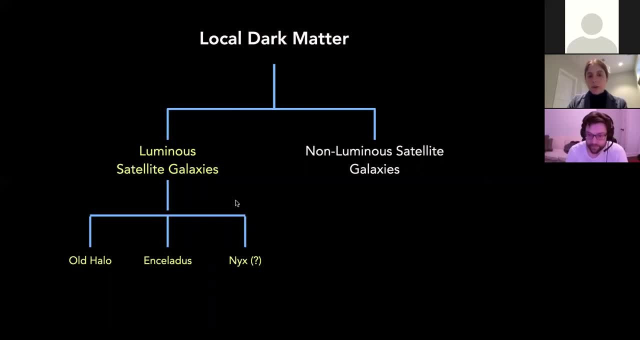 Anna Voelker. So this new result here with Nix is filling in a new part here of the puzzle. There's a question mark because we have yet to confirm, Anna Voelker, Whether or not it really is going to be correlated with the local dark matter disk. 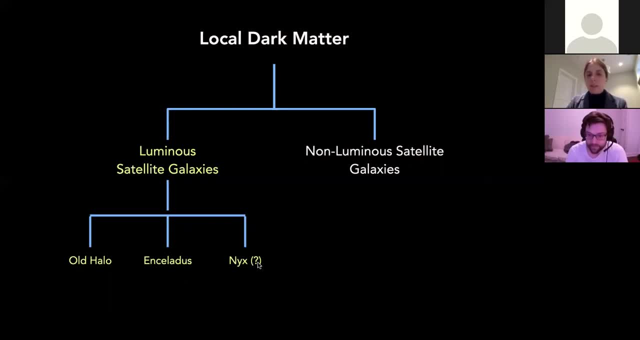 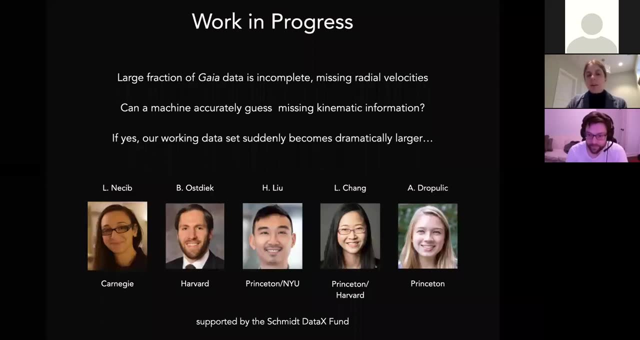 Anna Voelker, And that's something that we'll should be able to answer within the next year, Anna Voelker. And just to mention very briefly some work that we have going on in progress with a large group of postdocs and students at Princeton. 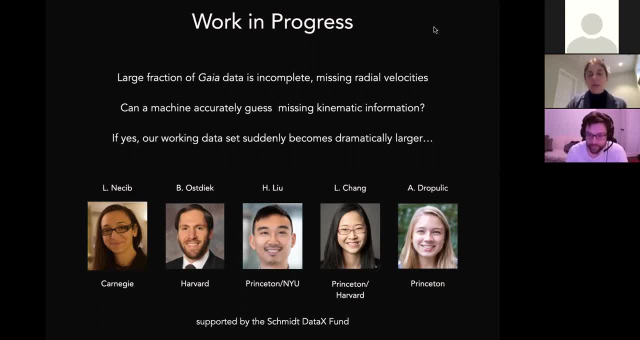 Anna Voelker In moving this forward and trying to maximize the amount of information that we can get from the Gaia data. Anna Voelker, You know, everything I've told you is just using the small subset of Gaia data that actually has full three dimensional volume. 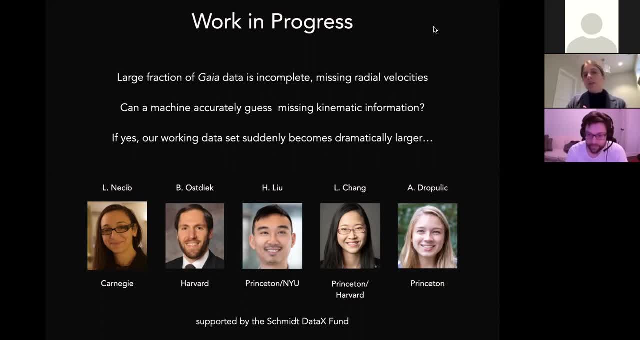 Anna Voelker And that's a lot of velocity information, but there's an even larger fraction of the Gaia data. that is, Anna Voelker, Missing some of that velocity information and, in particular, missing the line of sight velocity. 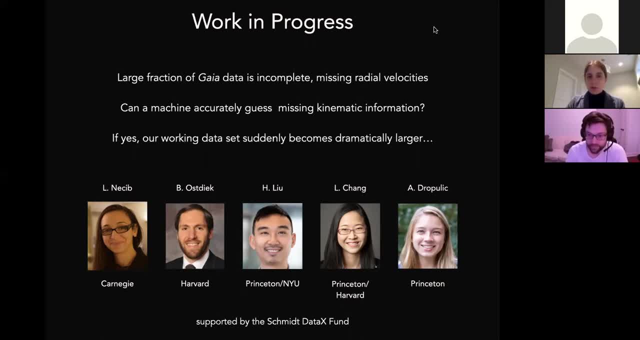 Anna Voelker. So one of the things we're working on now is asking whether or not we can use regression neural networks to actually guess what that missing kinematic piece of information is, Anna Voelker, And if that neural network approach works successfully, then that would allow us to. it would greatly expand the working data that we can. 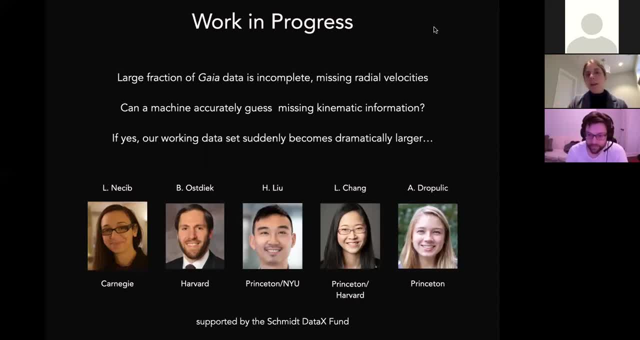 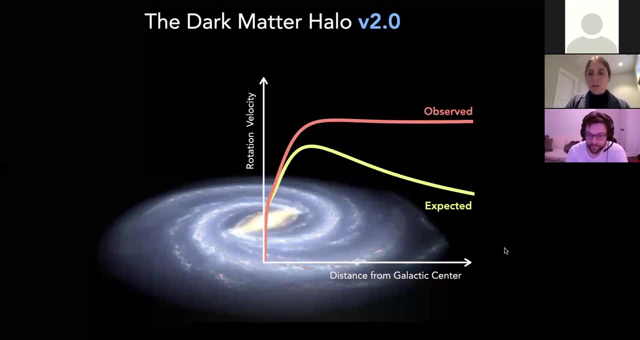 Anna Voelker. Look at to Anna Voelker, Find you know to do clustering and find evidence for for these mergers, Anna Voelker. So with that, I'll just conclude by starting where we, by going back to where we began. so 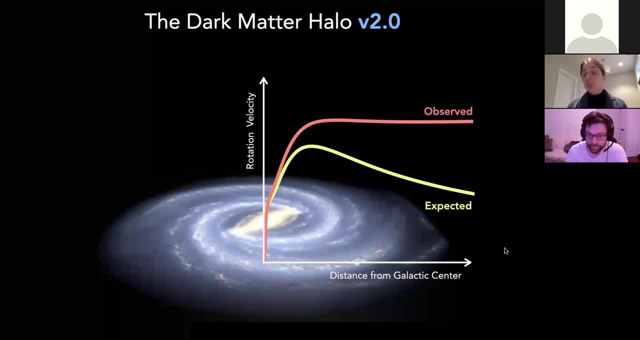 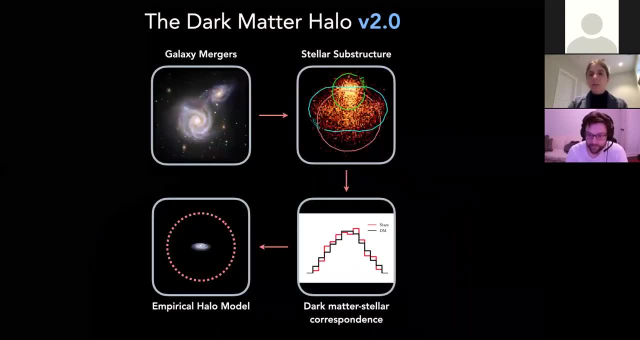 Anna Voelker. When the start of the talk, I presented our initial picture of what the dark matter distribution, our galaxy, look like, which was based off of observations from the flat rotation curves, Anna Voelker, But with the new data that's been coming from Gaia, 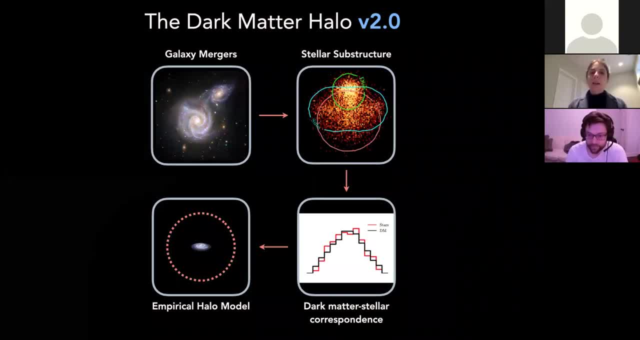 Anna Voelker. It's allowed us to revisit that and by using information about stellar substructure, combining that with what we're learning from state of the art and numerical simulations about the correlations between stellar distributions and dark matter, we can piece that all together to build up an empirical model for the halo.